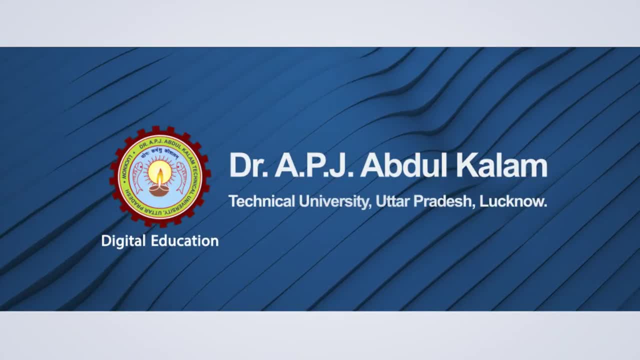 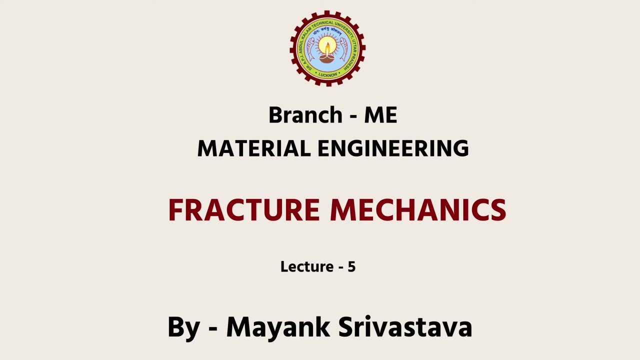 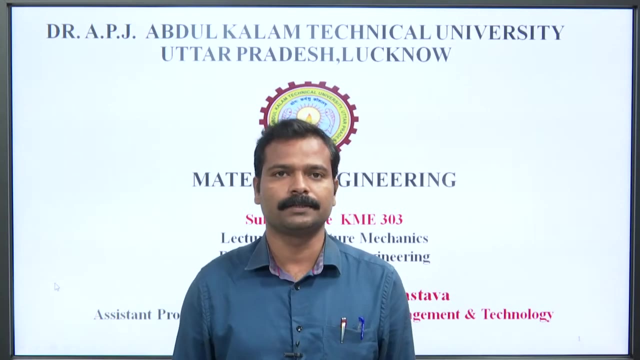 Hello friends, myself Mayank Srivastav, from Mechanical Engineering Department of Ambalika Institute of Management and Technology, which is affiliated with Dr APJ Abdul Kalam Technical University, And today I am going to teach you a mechanical engineering subject material. 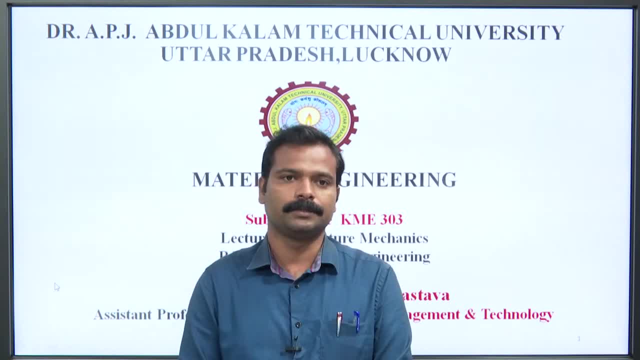 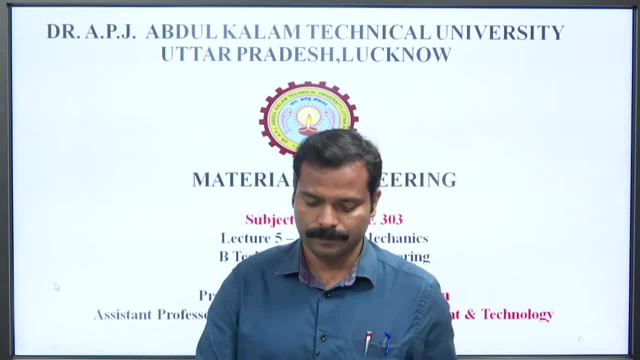 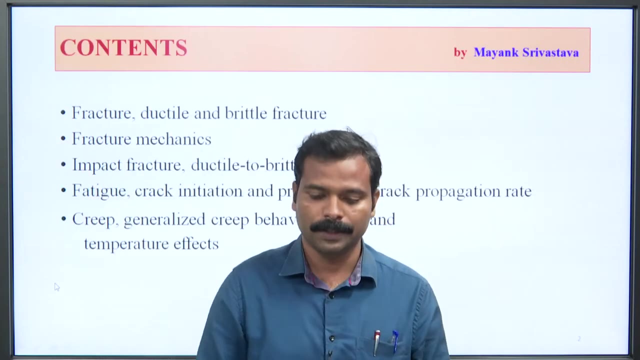 engineering subject which is subject code is KME 303, which is used in the second year and third semester. It is normally taught. So today's topic is our fracture mechanics. Today's topic is our fracture mechanics. Actually, as you had read in the previous lecture that 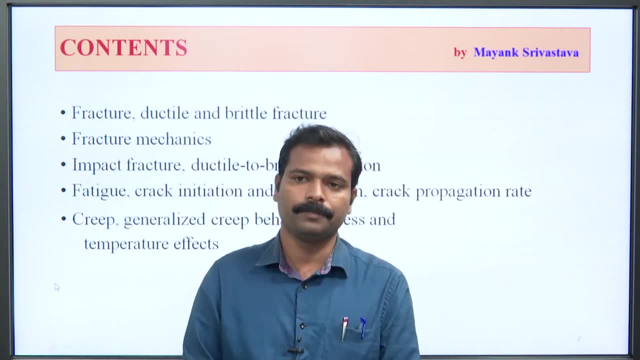 we had told the theory of failure. What are the things in the theory of failure? that any thing or any design or any material of yours fails. So a theory was given for that. Now, according to those theories, now in this lecture you have to read when the material is fractured: 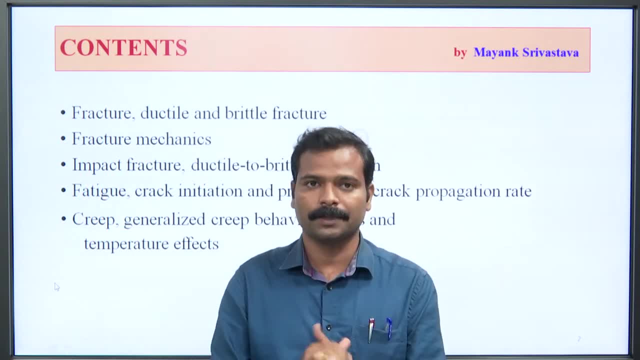 and what are the trends of its fracture? Fracture trends means if it comes on your trends, then like if you have wood now, if you impact on wood, then whatever fracture will happen. or fracture means separation of a single body into two different parts. 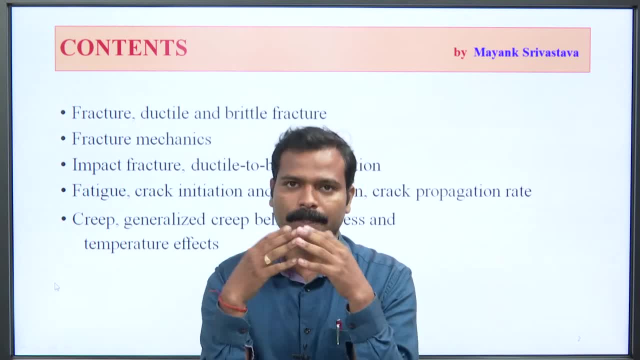 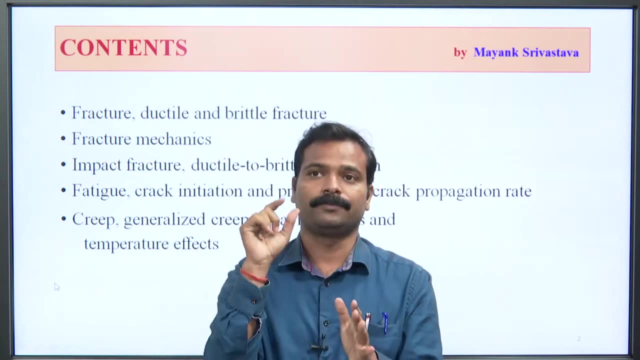 If you divide a single body into two different parts, or it breaks due to an impact or due to a load, then you call it a fracture. So now the fracture trends you have to understand, like if you have wood with wood, if you impact on wood then it will break, or the tendency. 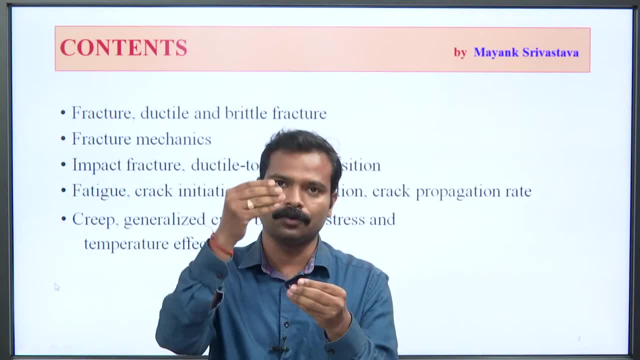 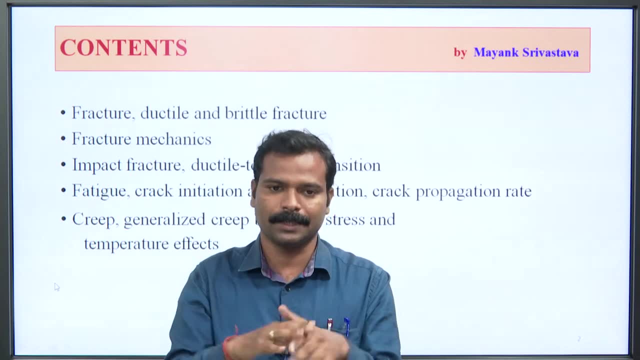 to get its rapture will differ from that of another material. Like if you talk about your universe or you talk about the language of your engineering or your engineering science, then it will differ from that of another material on the other side, like you speak about the 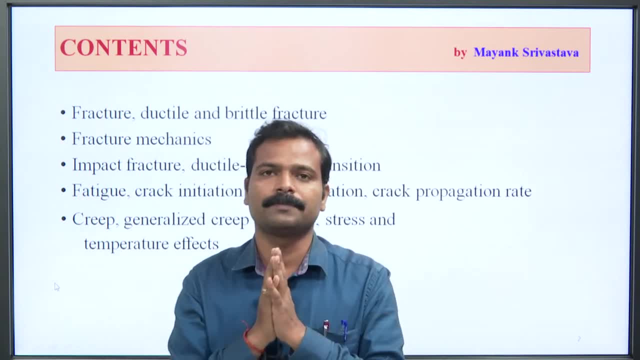 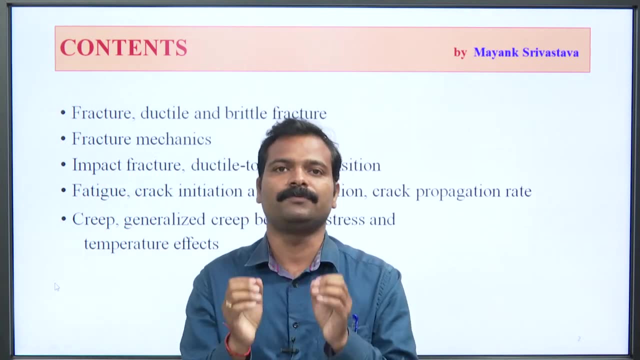 language of your engineering or the science of engineering or your theory is not about: If you load all the materials in it, then at some point there will be a fracture, at some point there will be deflection, at some point there will be failure. 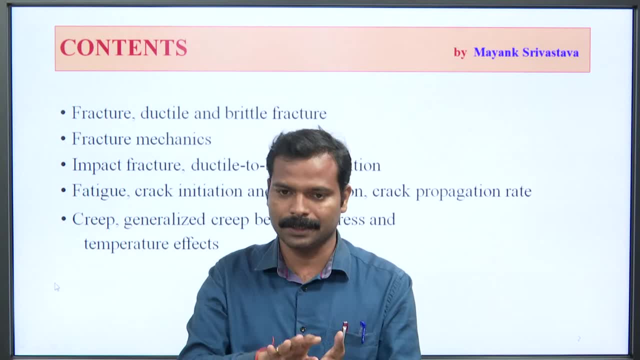 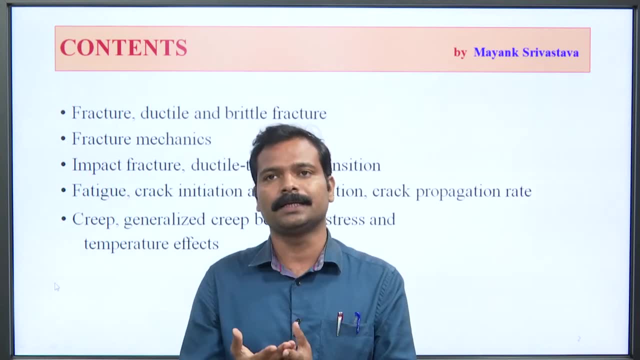 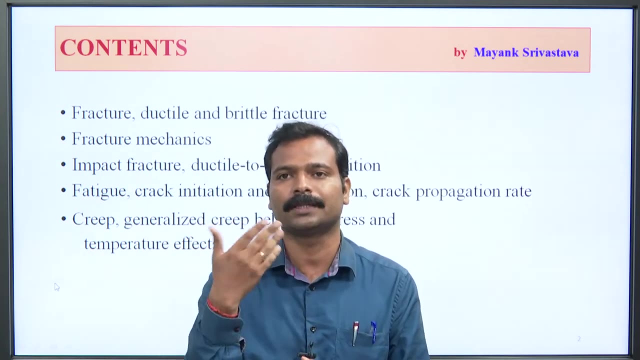 So why will there be failure? How safe is it? In which region is the current failure happening? That was explained to you in theory, But the tendency of failure is that how will that failure happen? And the most important term is that, how will the failure happen? What will be the failure following? 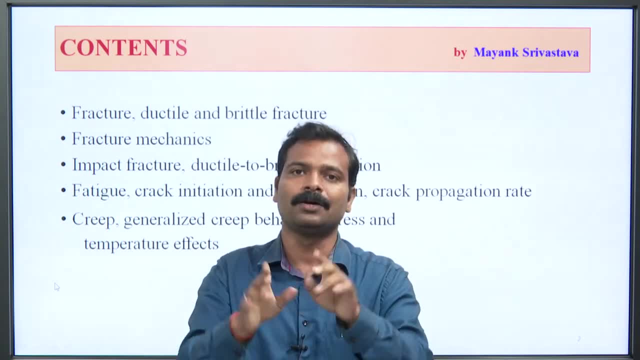 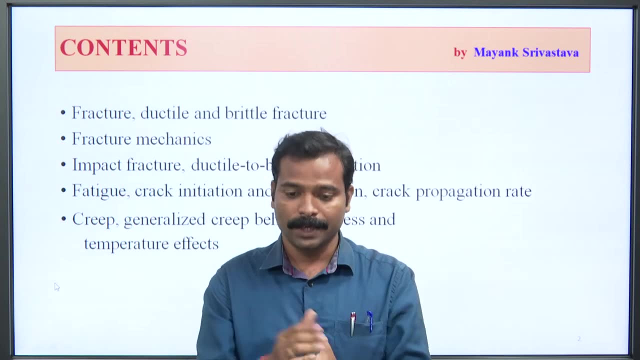 Or when the failure happens on its outer surface, then what will be the tendency of the cut section part, Or how will it look? So all these things you read in fracture mechanism. Before coming to the topic, let us tell you the terms that. why did it come? Where did it come from? 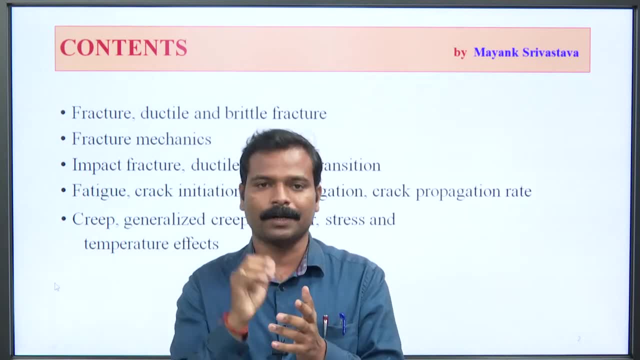 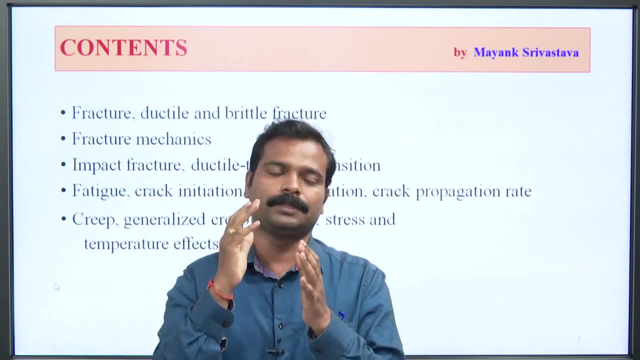 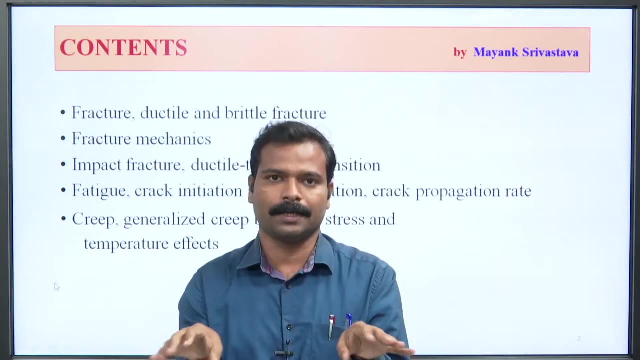 Fatigue is a word, Fatigue. How did fatigue come in the market? When did people understand it? Actually, what happened in the 1880s Once? there was a train that was moving on its track at a very high speed, So suddenly, what happened in it? its front axle broke. 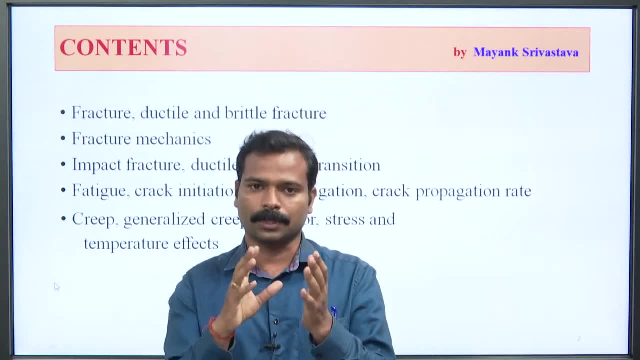 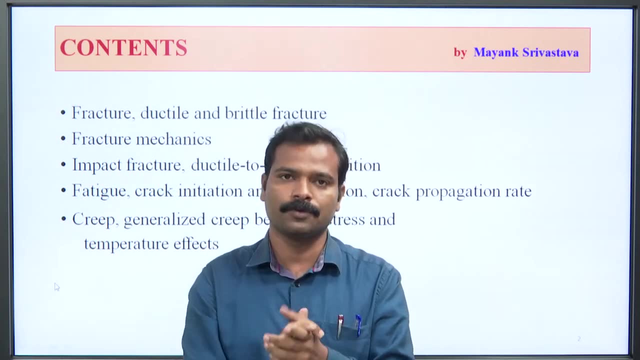 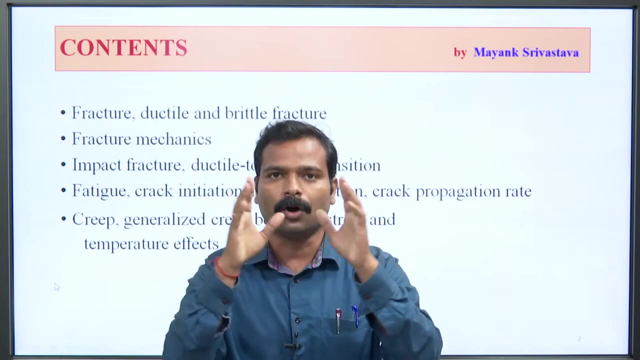 And when it broke, when its nature was seen, it was ductile, But the nature that it reflected on breaking it did as a brittle. As a brittle means there was no plastic deformation in it, It broke. When ductile material breaks, then your shape changes and takes time. 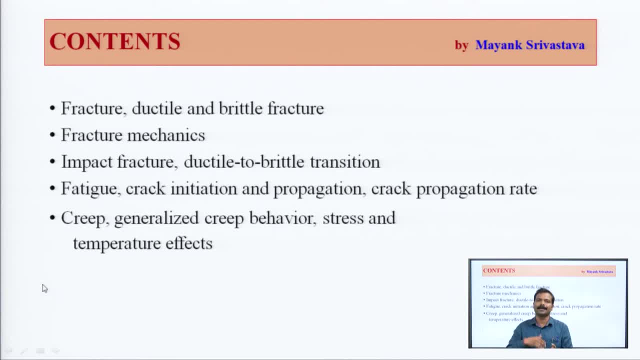 But brittle. If we talk about brittle material then it directly shows your fracture. So when all these things were seen in it in the 1880s, So the first fatigue terms came in people's knowledge that why did it fail? So it came to know that it failed because of fatigue. 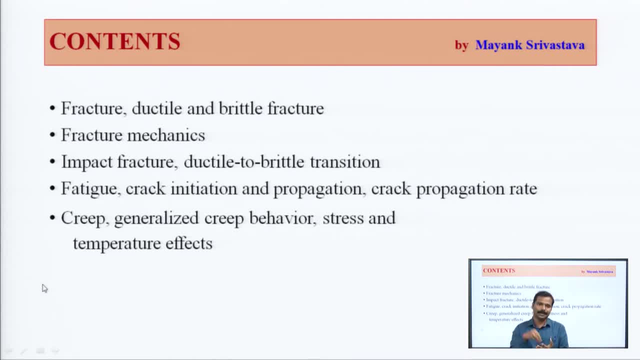 What are fatigues? Fatigue is your cyclic loading or repeated loading. Suppose there is anything, suppose it was an axle, If the axle is made or it has been developed in any part. So if there is a little bit or a small amount of your pit or one of your voids or cavity has been left. 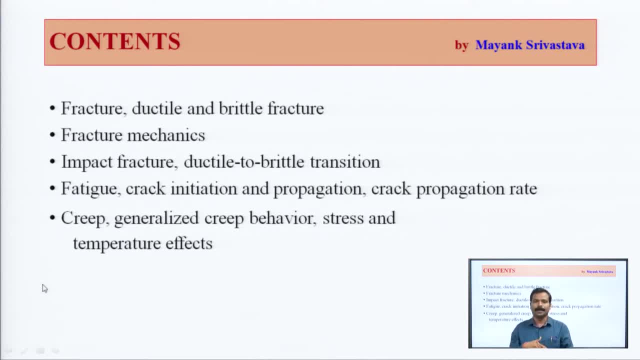 Or there is a little porosity left. So what happens in it If there is cyclic loading or repeated loading? Now suppose this train is running again and again. Because it is a train, it will run. So when it is running again and again, what is happening in it? 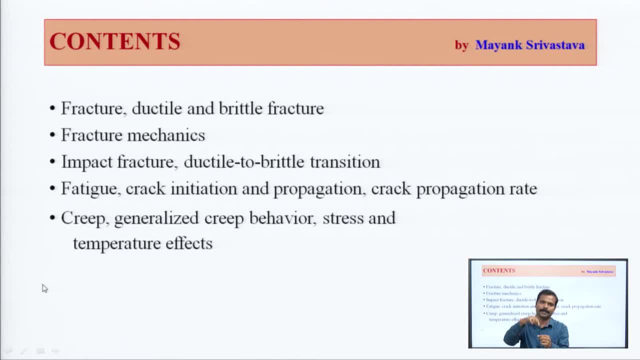 The load is being impacted there again and again. So whenever the load is being impacted at the same place or on the axle And there is already a very small void there Or there was a very small impact. So what does that thing do? 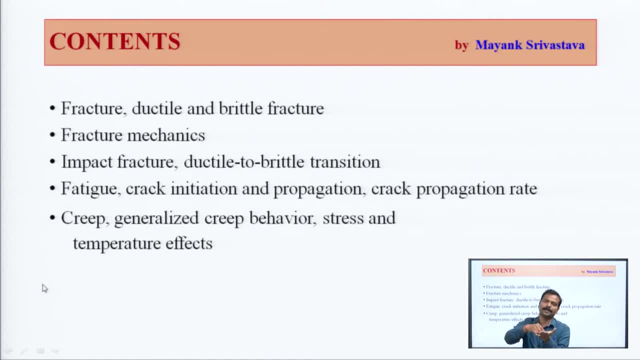 What happens in a longer period of time? Slowly, slowly, slowly. when it will be a repeated load, There will be a cyclic process. So what will it do? slowly, It will increase it. So this process happened in the case of the train. 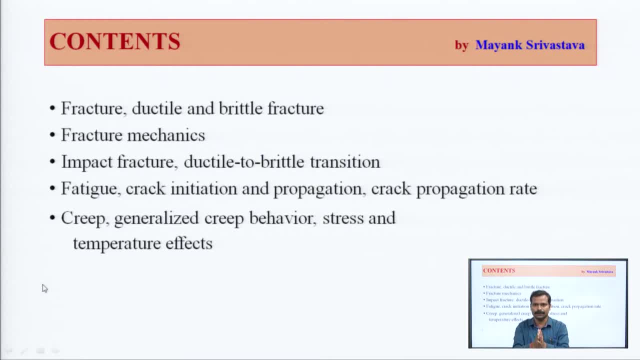 It kept increasing it And suddenly, what happened? It failed. And when it failed, we thought that it should have been like ductile Means: your elongation should have been, Neck formation should have been, Cavity should have been And grain growth should have been. 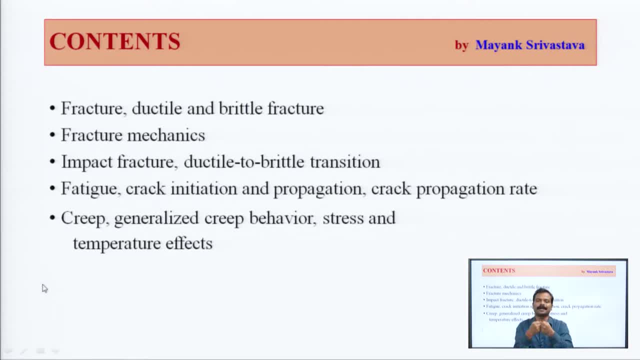 But there was no grain growth in it. Sudden grain came out. Now what does grain mean? to come out, Or detached, If you say in the engineering language. Actually, if any part is made, So basically if that is seen, Then it is made together with the grain structure. 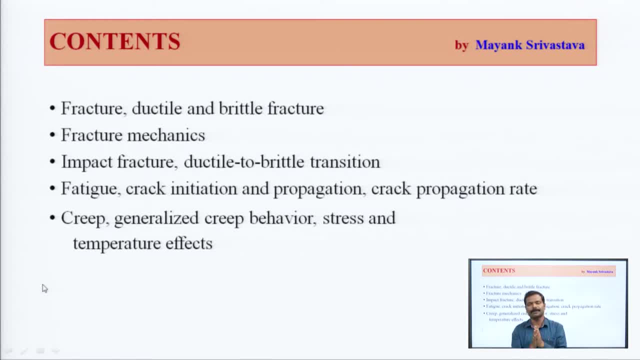 If there is anything in any universe, If we talk about our body, then it has a grain structure. Or if we talk about metals, then they have their own grain structure. So the atomic bonding of the grain structure, Or the bonding or packing. 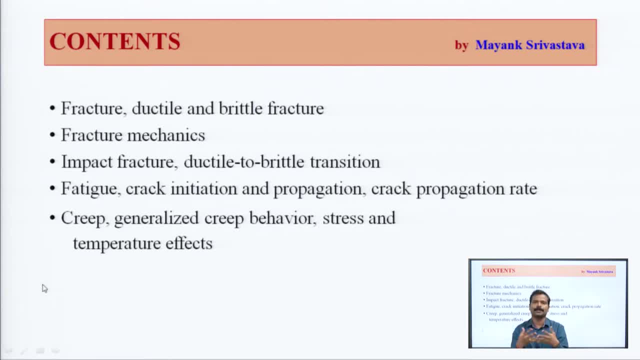 All these things depend on it. The better the bonding, the less the chances of failure. But if the case of brittle is seen, then it is hard, But the ductile quality is not there in it. Now what we have to study in today's content. 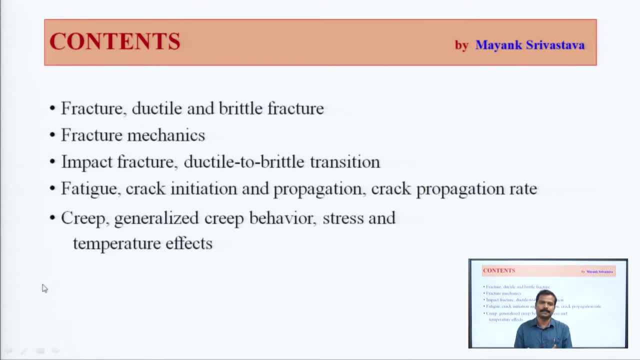 This is the fracture. What is fracture? We have told the fracture A body, A single body which, when external force is applied on it And it will be break into two different parts, Then it is known as a Fracture. 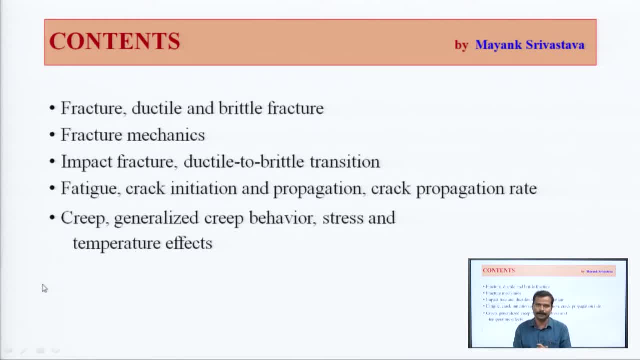 Now the second is ductile and brittle fracture. You have to study further in this. Then what are the things of fracture mechanism? Why fracture mechanism is important? This is most important from design factor, If you do not know when any material will have fracture. 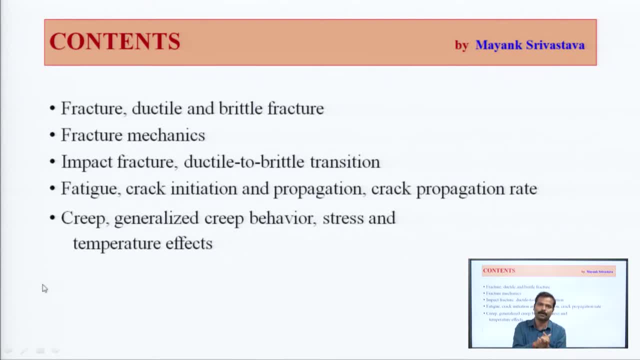 What will be its tendency? Then you will not be able to cover it up, You will not be able to design it safely. So what do you do to avoid all those things? We study about fracture mechanism. Now comes the impact: fracture or ductile to brittle transmission. 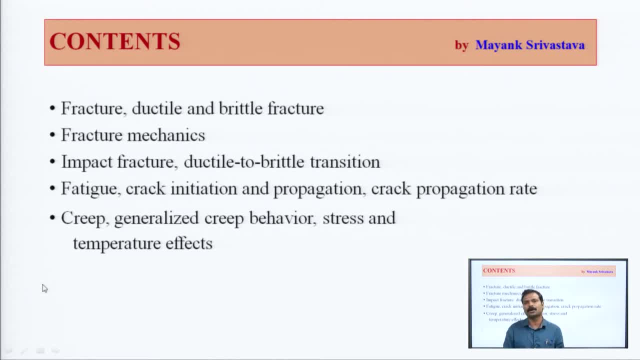 What will be the impact on fracture And ductile to brittle? How does it have transition or phase transfer? Then fatigue Or crack, initiation and propagation And crack propagation rate. What we have told you about fatigue: Because of cyclic loading, Fatigue, failure occurs. 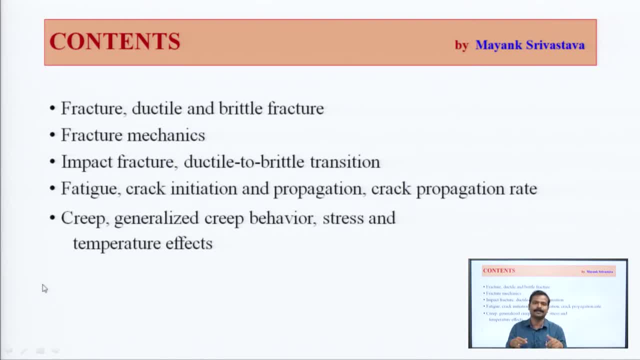 Repeated loading occurs Because of that Example. For example, Cycle, Bicycle: You ride it. So when you ride a bicycle, So its pedal, You give more or less pressure, But one cycle. But it is a cyclic cycle process. 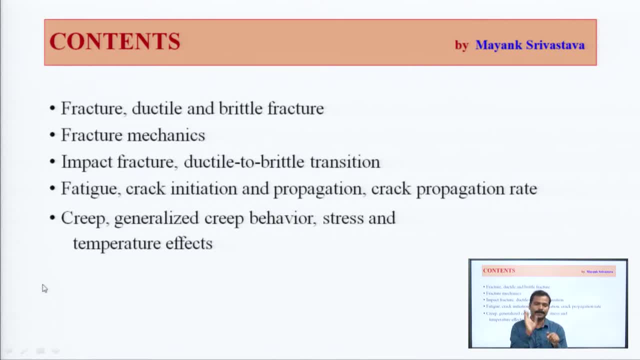 So in that case, Again and again load comes on it. So that is also an example of fatigue. It is repeated load. That is also an example of fatigue. Or talk about its handle If you ride, For example When you go to some dump or pits. 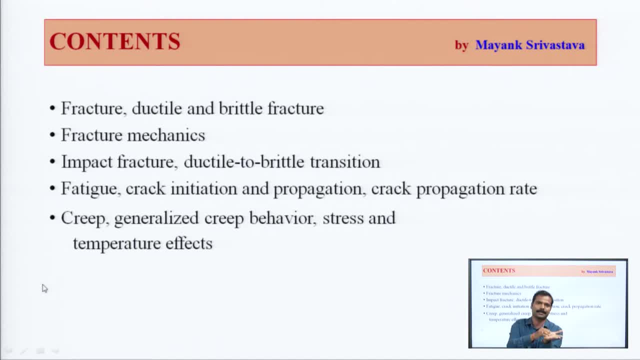 So what happens again and again? What happens on its handle Again and again? shocks come, Or vibration comes again and again. So that is a cyclic process. That is why we think It is very easy to design anything, But before launching any product in the market, 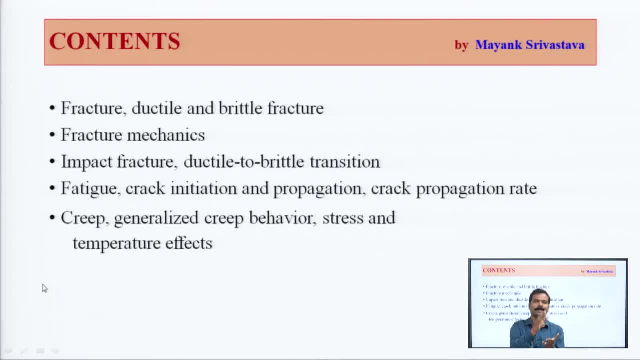 There is a lot of testing on it, So in them too, This cyclic process plays a very important role. Now comes the crack initiation. How crack develops- We will study this further- How propagation happens in it Means if, once the crack develops, 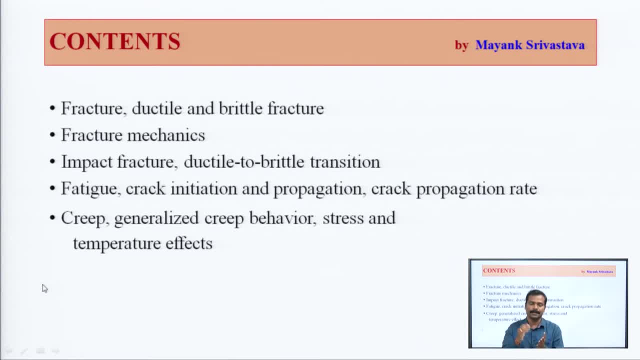 Then why does it propagate? Propagate means increase Means. with respect to time, It will be increased And crack propagation. What is the rate? How much impact will there be? So at what rate will it change? So we will study about this. 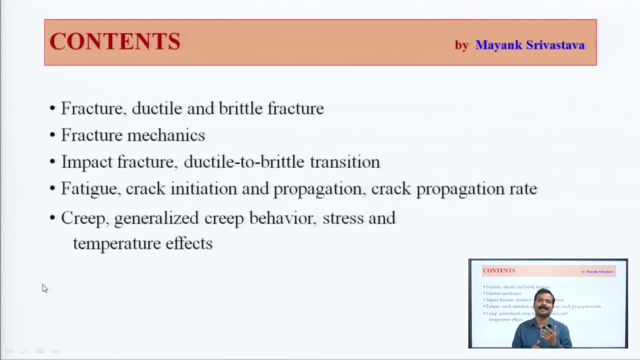 Then comes the creep. Now like creep. What is the generalized creep behavior? We will study about this. What is the stress and temperature effect? We will study about this on the material. But we will explain you creep first. What is creep? 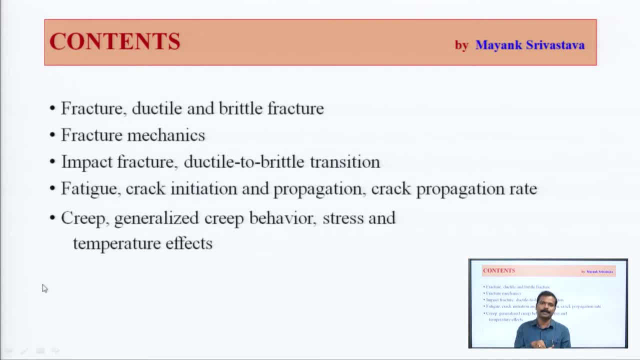 That a constant load is applied on any body For a longer period of time Means if there is any body of yours, If any load is applied on it And apply for a long time And apply constant load, Then it is creep. 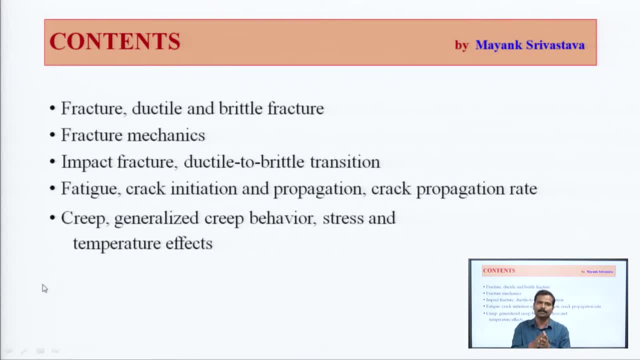 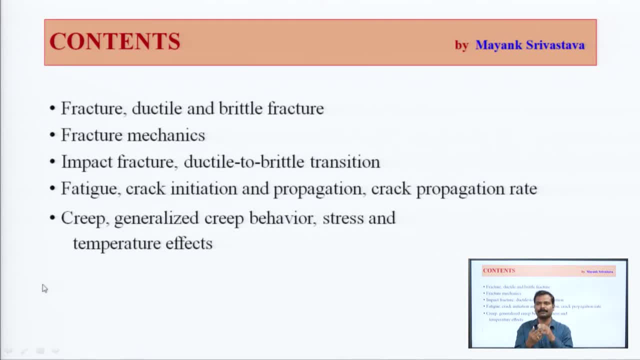 Then it is called constant load. We think that it is so less. But when that load is applied, Then longer period of time, After 100 years, 200 years, What happens in that Failure starts to come. So what happens? 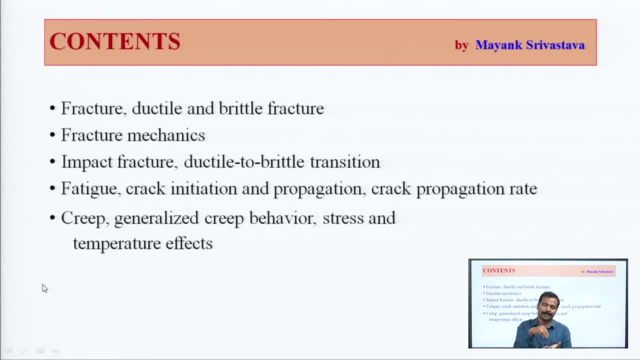 It is called creep. Why? Because constant load is applied, But with respect to longer time, It is taking more time. So whatever failure comes in it That you call creep, Let's move to the next slide. Failure of material components is the loss of ability to function normally. 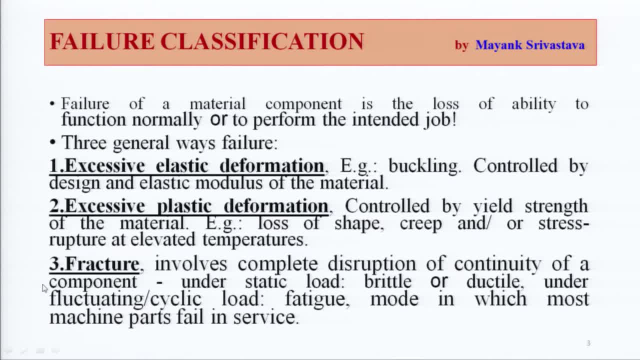 Or to perform the indent job. If we talk about failure, What is failure? What does it mean? Whatever the design is, Or any mechanical component design, So it has some life Or it has some job. That, yes, It has to work for so long. 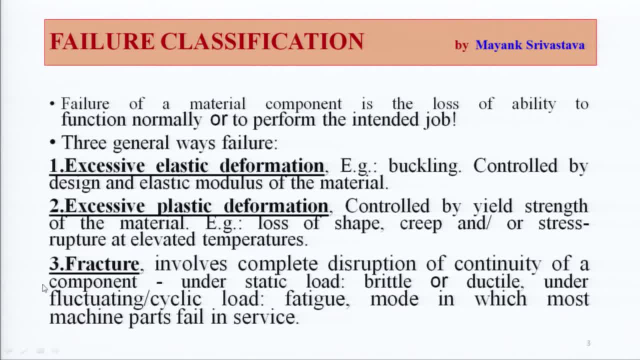 Or it has this ability, But if it fails To perform its 100% Or its ability, So that is what you call failure, Failure of material. Now there are three general ways of failure, Three general processes, Three general ways of failure. 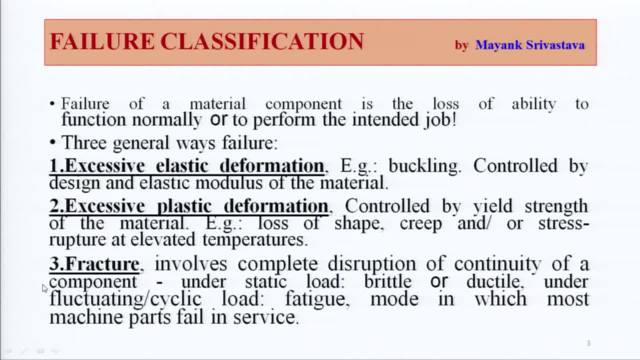 The first, The second, The third, The third, The fourth, The fifth, The fifth, The sixth, The sixth, The seventh, The eighth. So there are three general processes, Three general processes Because of which any material Your 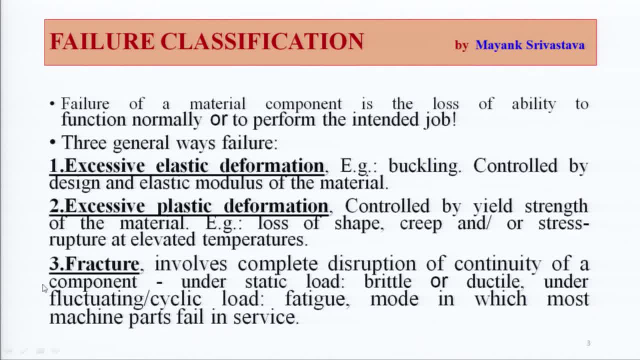 Failure. First is Excessive elastic deformation, Elastic. I have told you in the previous lecture What happens in elastic, That stress And strain Same And What is the quality Any material In its elastic limit, Say when it regains? 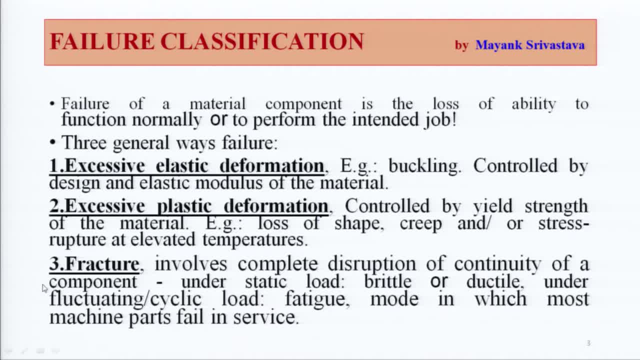 The shape Means if in it Stress, Stress Involving Or stress Coming. So in that case What happens? deflection should also be the same. suppose you have applied tensile force on any particle. when you are applying tensile force, 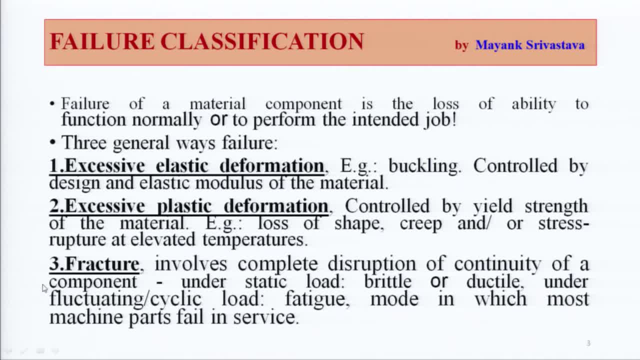 so how much it will deform that with respect to the stress which is being developed in it. so this is your elastic. if this thing regains, leave it and take its shape, then we will say in elastic range. but what is the case here? when the failure will happen. 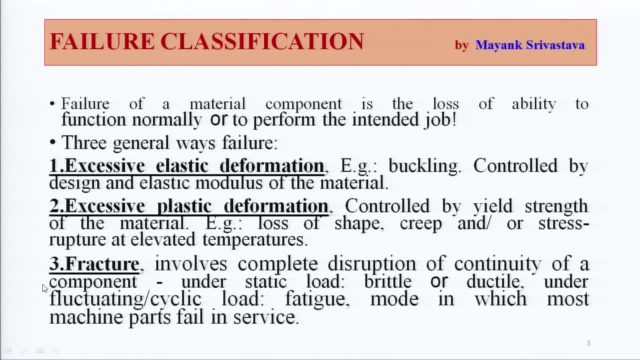 when it will cross the elastic range, there will be deformation- example: buckling- controlled by the design and elastic modulus of material. second, let us talk about excessive plastic deformation. now, what is plastic deformation? permanent deformation, you can call it plastic deformation. plastic deformation means it cannot regain its shape. 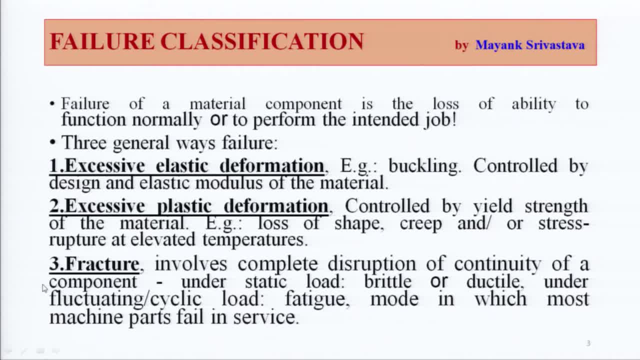 once deformation is done, it cannot regain its shape. now let us control it. control by yield strength of a material. we call it stress creep and stress rapture at elevated temperature. now, in this also there is a role of temperature. suppose if we are giving temperature to any material. 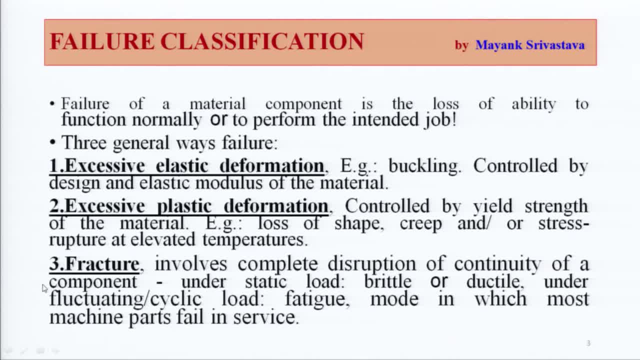 then its grain size will change. now, what does grain size change mean? any matter in the universe or any material. it is made of two things. one is matter and another is energy. now, what things come in matter, like solid liquid and gas. now, who do you call solid? 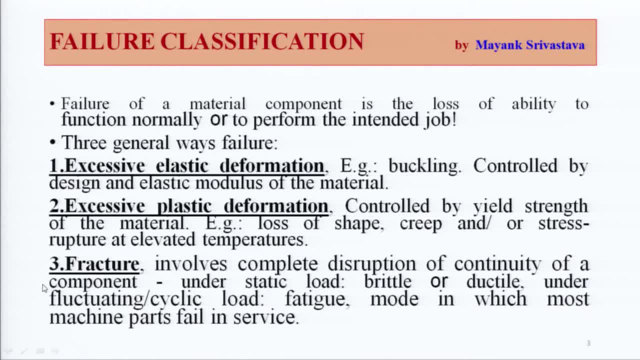 So in that case what will happen is that the phase is changing and it is leaving its grain structure. So if the same process of grain propagates slowly or leaves it slowly, then you can say it in ductile material. But if the grain leaves its atomic bonding together, then it comes into brittleness. 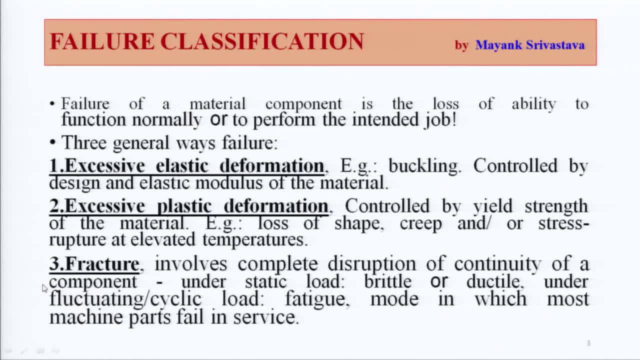 What is your third point? Fracture. Fracture involves complete disruption of a continuity of a component under static load. Now, we had already told you about static load. What is static load? It is a constant or equilibrium condition in which the net value should be zero. 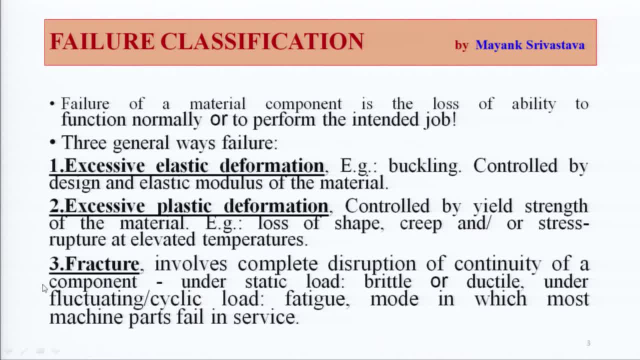 Of ductile under a fluctuating cyclic. Now look at the same cyclic. in this It is a matter of fatigue Mode in which most machine parts fail. That is why most of the components or moving parts of the machine fail. It will be due to either static load or due to dynamic load. 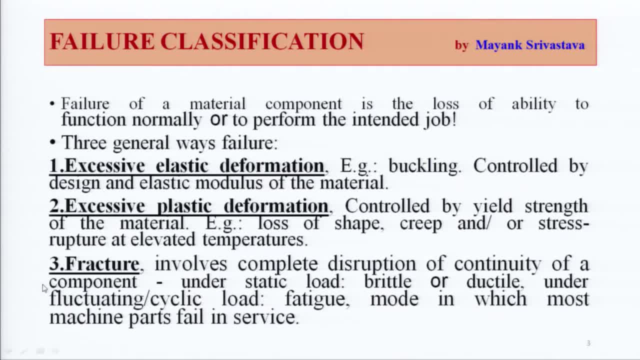 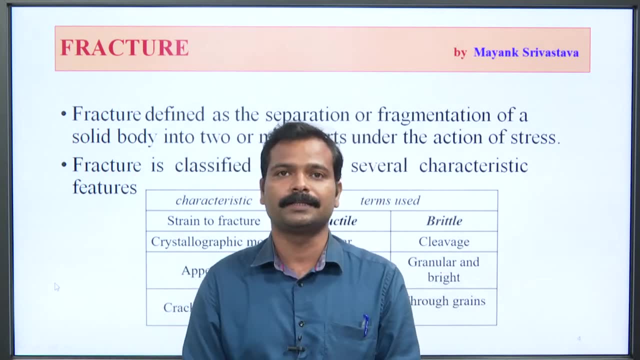 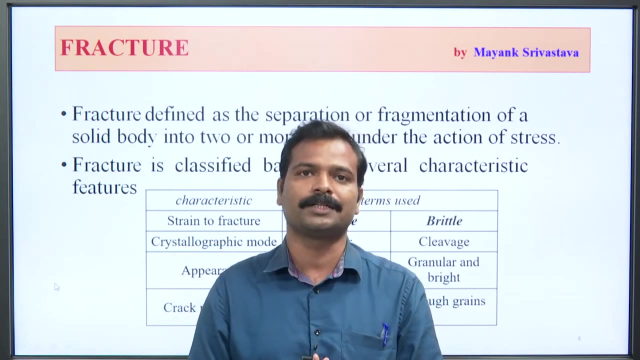 And in dynamic you get cyclic or repeated load, Or we talk about fatigue and creep. So these are the three types of criteria due to which your chances of failure increase. Now it comes to fracture, defined as the separation or fragmentation of a solid body into two or more parts under action of stress. 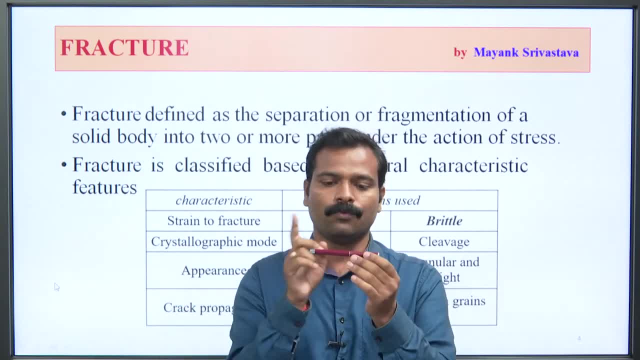 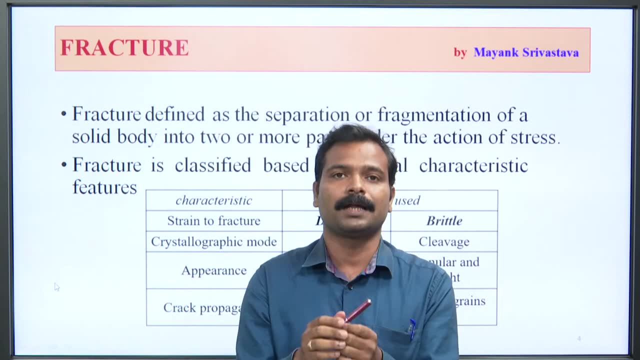 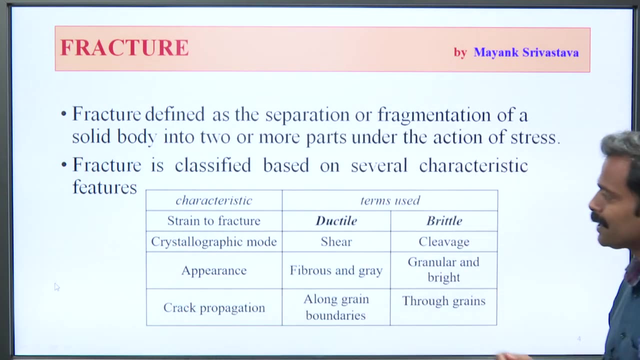 Means due to stress. if any one body breaks in two parts, then it is called fracture. Now, how is fracture classified? Fracture and classified are basically several characteristic features based on which it is classified. Now, as you can see in this characteristics and term used, 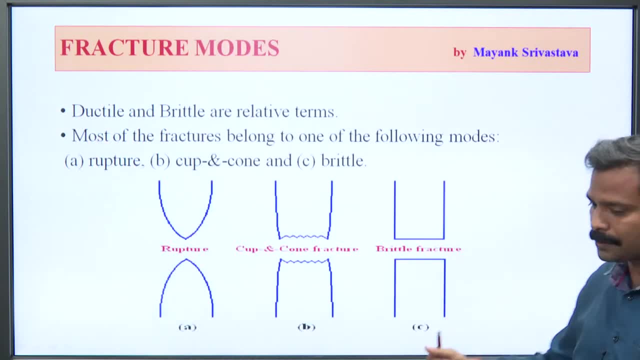 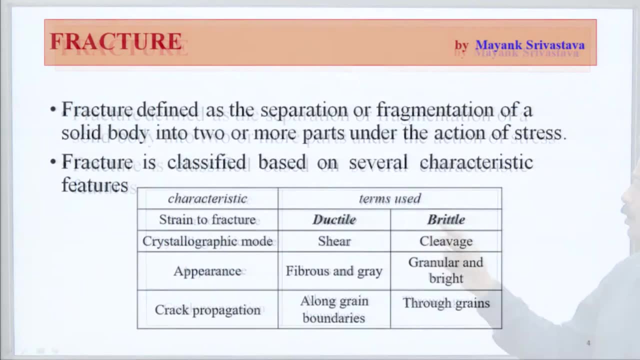 What are the characteristics of it and what terms are used in it? Now, strain to fracture, Ductile and brittle. This term will be used in strain, ductile and brittle. Now what is crystallography mode? In ductile, if there is a fracture in the shear mode, then it is called crystallography mode. 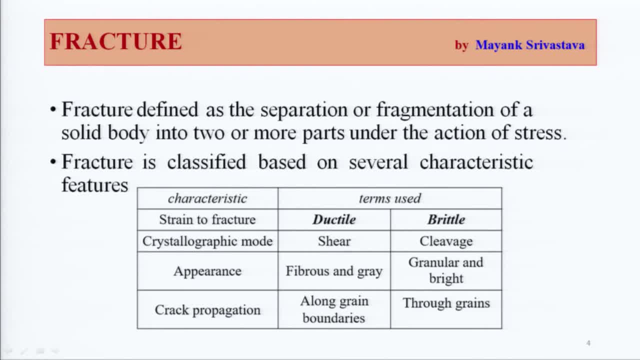 And in brittle what happens is that grains are left together. There is no bonding between them, So that is also called cleavage. After that comes appearance Fibrous and gray. Whenever there is a fracture in ductile material, then fibrous. 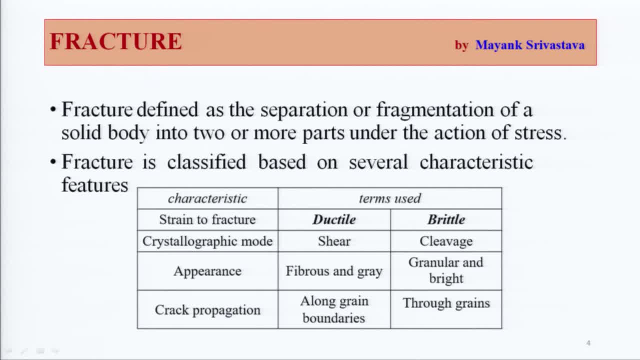 Fibrous means it will be in the form of fibers. It is not that grains will be left together. There will be neck formation and deformation in it. The properties will change gradually And its color is gray. If there is a fracture in any ductile material, then where there is a fracture it is denoted by gray color. 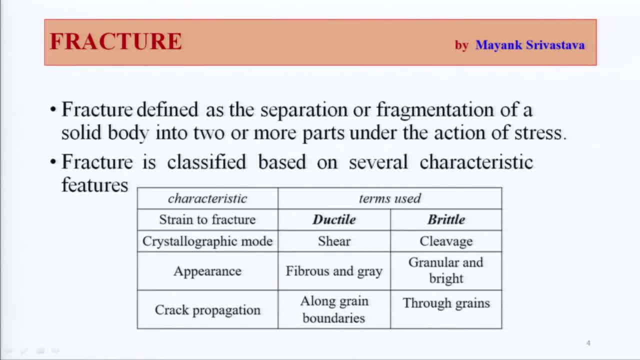 It is sewed by gray color. And if we talk about brittle, then granular and bright. Granular means it is in the form of grain structure, It is in the form of circular In the case of brittle, If you see the glass. if it breaks, then all the grains are separated. 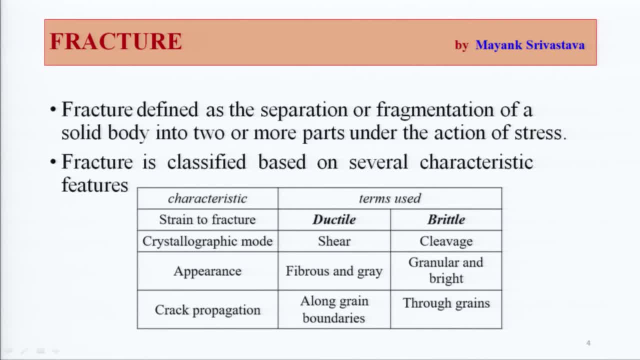 It is in the form of granular. There are no fibers in it. It is in the form of granular. And what happens? It is bright. Its color is bright to see. So that is the quality of your brittle. After that is your crack propagation. 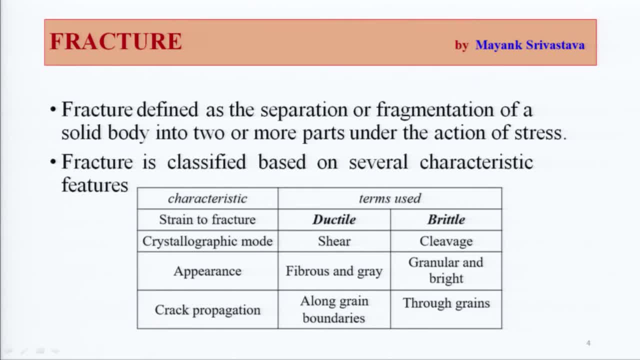 Now in ductile the crack propagates slowly Along grain boundaries. It will remain inside the grain boundary Along it. it propagates slowly. Now in the brief, when we show you the diagram further, then we will explain to you how it happens. 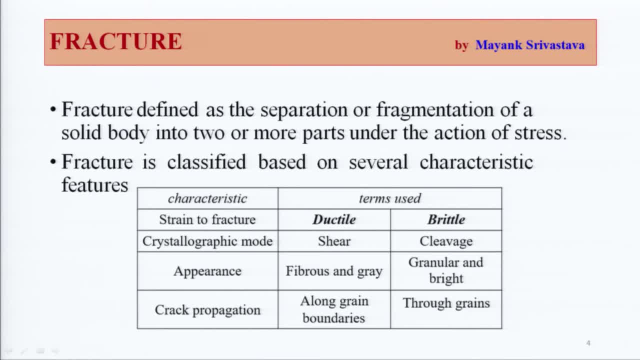 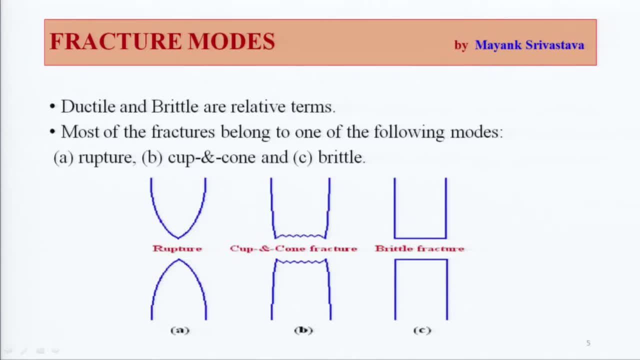 It happens within the boundary. And what happens in this? It happens through grains, Means, it happens throughout the grains, It is together in the whole. Ductile and brittle are relative terms, As we told you earlier that these two things contradict each other. 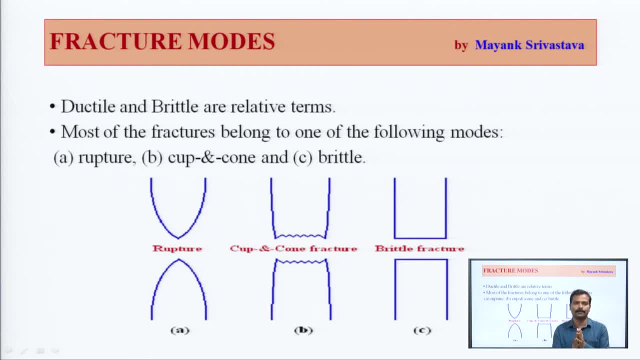 If the quality of ductility is in any material, then the quality of brittleness will be less, And if the quality of brittleness is in any material, then the quality of ductility will be less. For example, you can take ceramics. 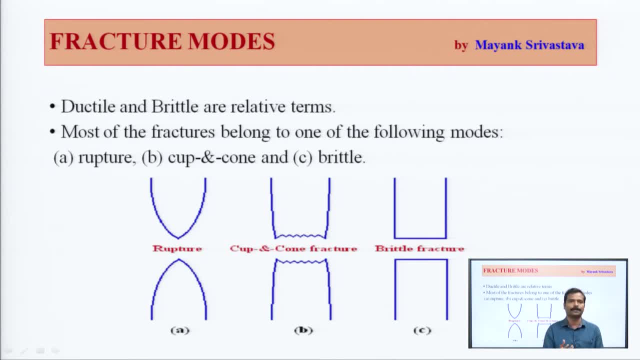 If you throw ceramics Or a cup like yours Which you use at home, If it is of ceramics Or tiles, If you have ceramics. So when you throw it, Or when it drops or falls from you, When it breaks, So what happens in that? 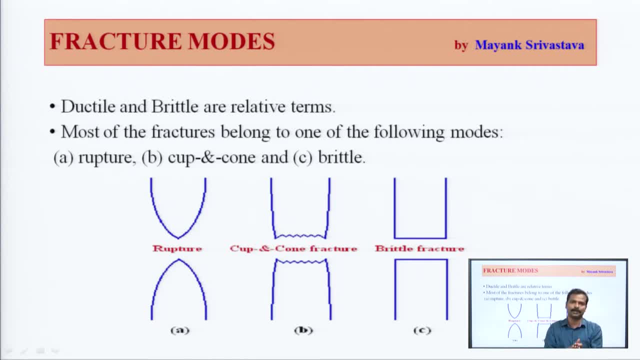 Brittleness quality happens. There is no plastic deformation from anywhere. There is sudden breaking. So that is the brittleness. quality Means ductility quality is less in it. Okay Now, after this, most of the fractures belong to one of the following modes: 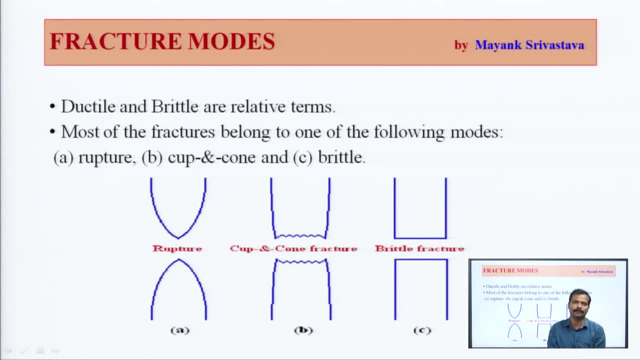 Now, all these fractures work on three modes: The first one, The second one, The third one, The fourth one, The fifth one, The fifth one, The sixth one, The sixth one, The seventh one, The sixth one, The seventh one. 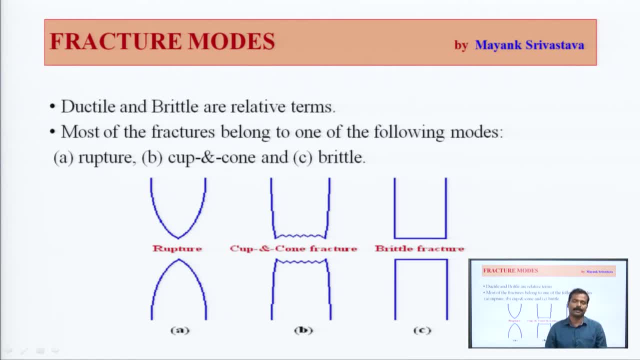 These three work on three modes. Mode one is rupture, Mode two is cup and cone fracture. And mode third is your brittle fracture. Now, if we talk about rupture, So in this, the grain structure, The grain size, You understand from its shape. 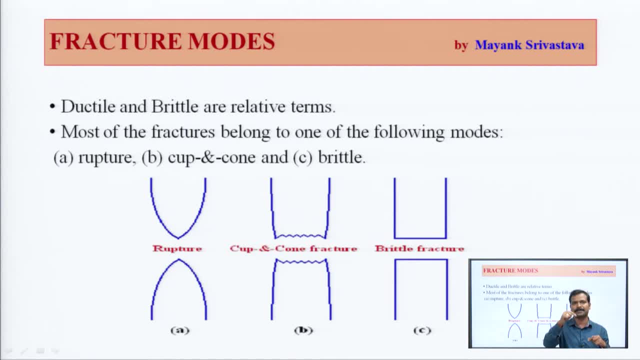 Which is taken in conical form, So the grain structure, When its bonding is there, When the atom breaks Or when it is loaded, Then what happens? It is slightly in long form Or in longitudinal direction, It grows up Or propagates. 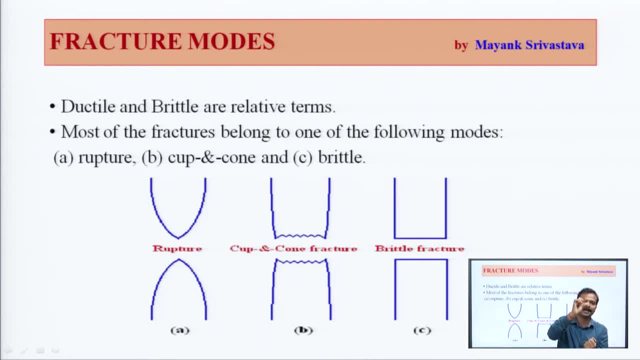 So its shape, It is taken by the neck formation, So it is called a neck formation. That is why we call it neck formation, So it is called a neck formation. That is why we call it neck formation, So it is called a neck formation. 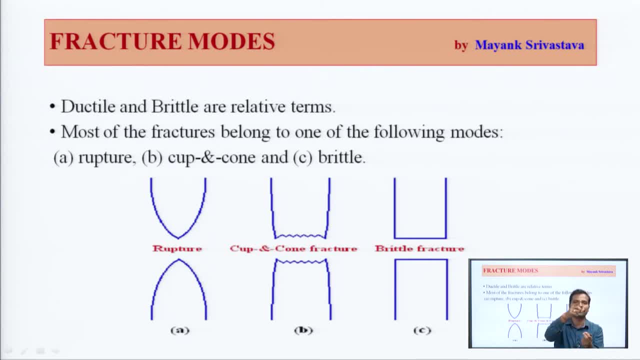 So it is called a neck formation, So it is called a rupture If these kind of qualities come there. And what happens in cup and cone fracture? If you see upper shape, So it is in cup form Whenever fracture is taking place. 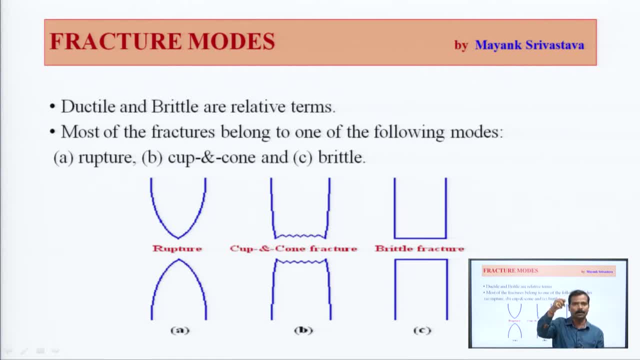 Now you have applied load again. So its shape came. It is in cup form And the shape below it is in cone form. So whatever fracture happens in it, It is in cup and cone form. Due to its shape, it is called cup and cone fracture. 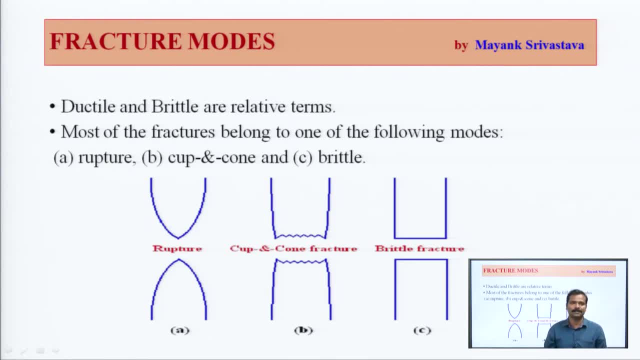 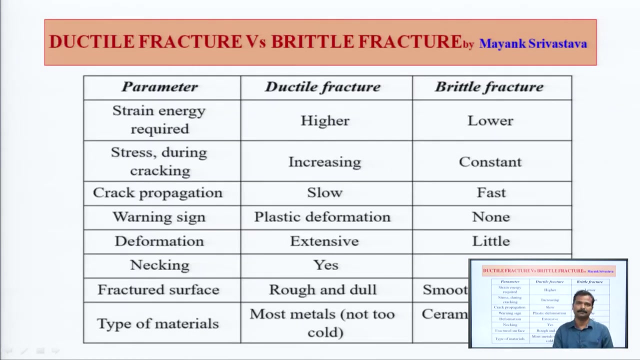 Now, in the first slide we told you about brittle fracture. What happens in brittle fracture? The atoms that are there- They are separate- suddenly propagate together, or there is no bounding left in it. that is why it is a straight line. This fracture shown here is a straight line fracture. 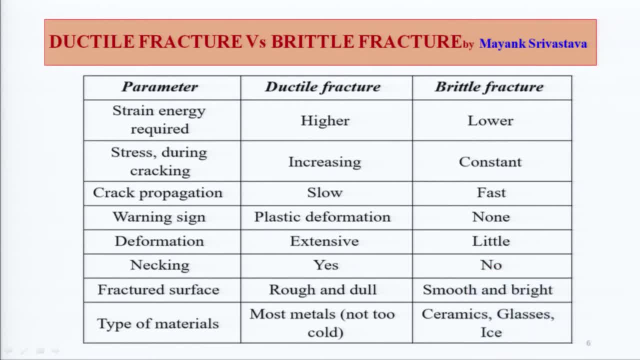 Now let's talk about the difference between ductile fracture and brittle fracture. What are the differences between ductile fracture and brittle fracture? What parameters should be considered if any material is to be tested in ductile fracture and in brittle fracture? So about this: one by one, we will explain to you strain energy required in the case of. 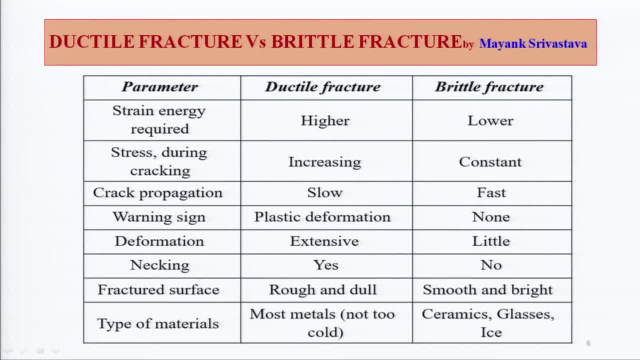 ductile. if any material is ductile, then strain energy is required in a higher amount, and if it is brittle, then it is required in a lower amount. Why does this happen? Why does it happen that in the case of ductile, higher strain energy is required and in the 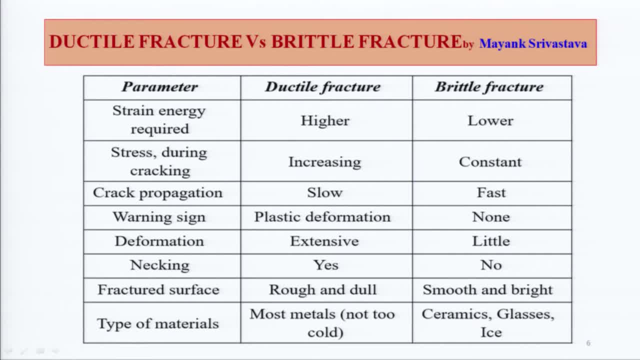 case of brittle, it is required in a lower amount. The reason for this is that, as we told you, in the stress strain curve this ductile material also follows the elastic limit and also follows the plastic limit, so it takes more time. That is why more energy is required. and what happens in the brittle material? there is direct plastic deformation, so it takes less time. and stress during cracking is always ductile fracture. So in the case of ductile fracture the stress required will be more. If you want to increase cracking, then the ductile material increases and the cracking 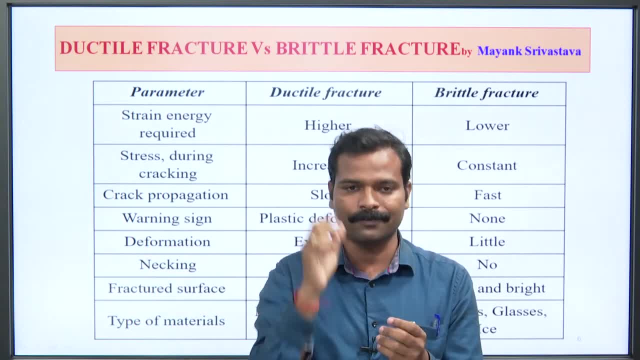 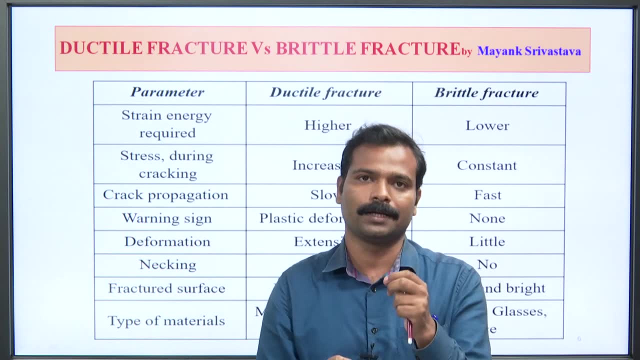 is done on the constant in the brittle material. Why is this done in the ductile Suppose? before the crack formation happened? now the time duration increased. then what happened? in that you will need more force to put the load, so in that case, the stress. 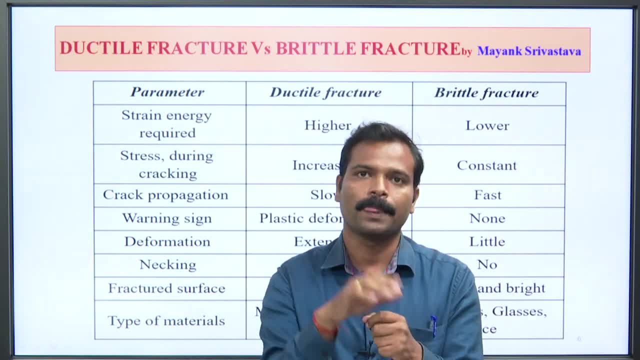 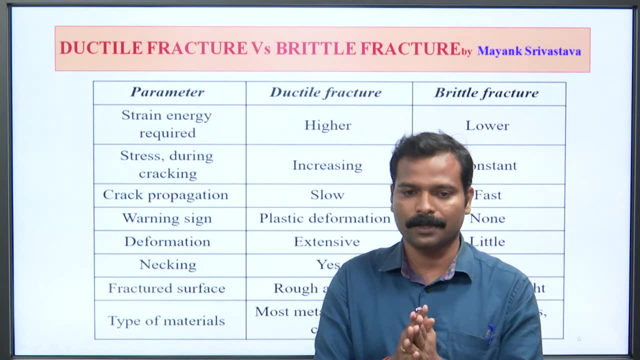 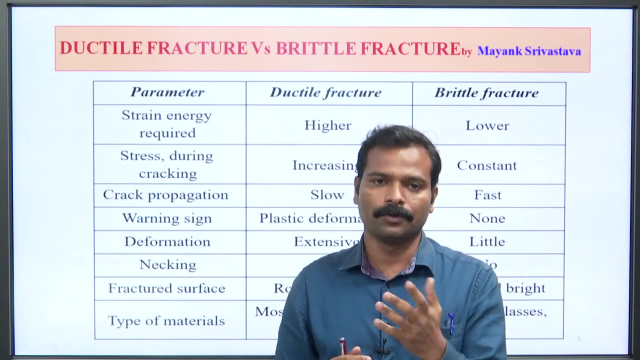 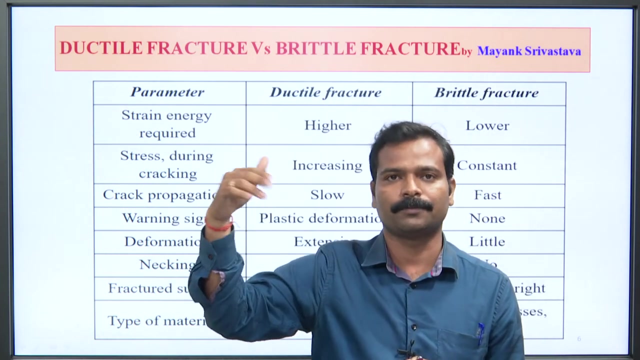 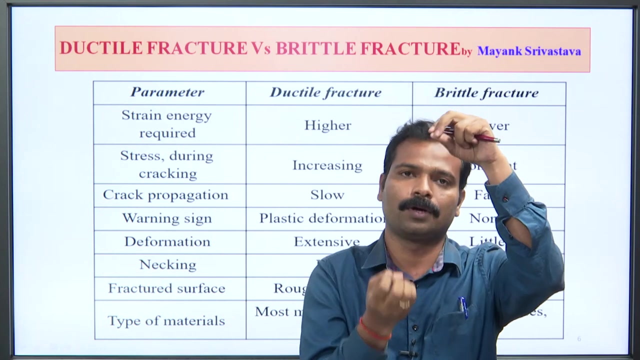 increases in cracking in the case of ductile and it does not increase in the case of brittle. Now the third point is crack propagation. if there is any ductile material, then if there are cracks in it, then those who propagate do it slowly. do it slowly because then it follows the same stress strain curve. first it will follow the elastic limit, then it will go to the plastic limit, then it will follow the upper point, lower point, then it takes time in it. the crack propagation is the crack that increases. you put pressure or load on both sides. now the crack is increasing. the crack that increases. it has to increase. 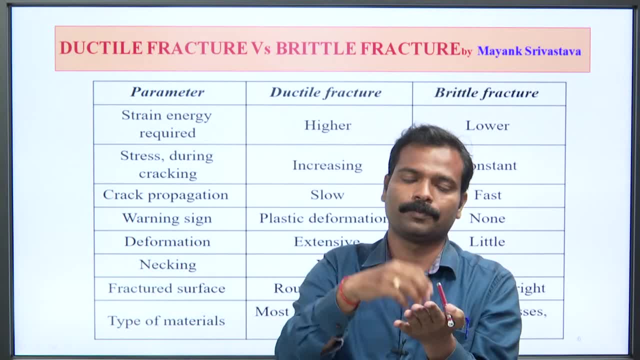 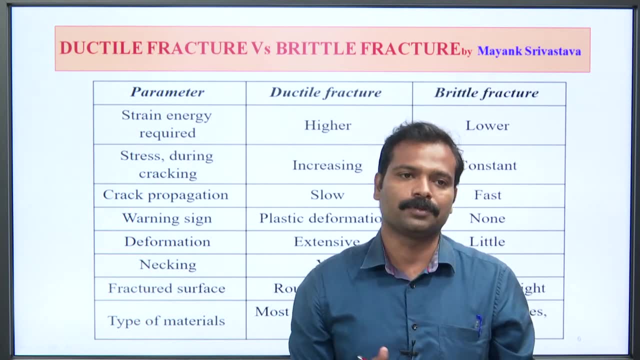 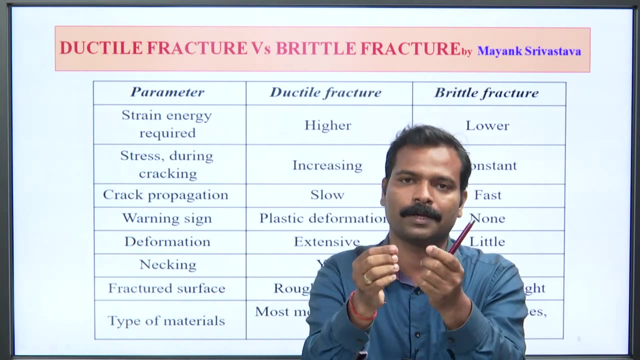 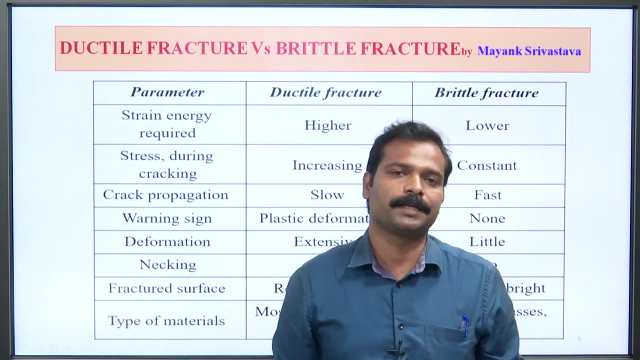 In case of ductile fracture. and what happens in brittle, it is very fast. you will never see that there is any material of brittle material or glass, then first a slight crack came, then it increased a little, then it increased a little, then it broke. it does not happen like this. what comes in it, direct fracture, comes okay. in this next parameter it is also very important that warning sign. if seen in an industrial use, then it is very important. 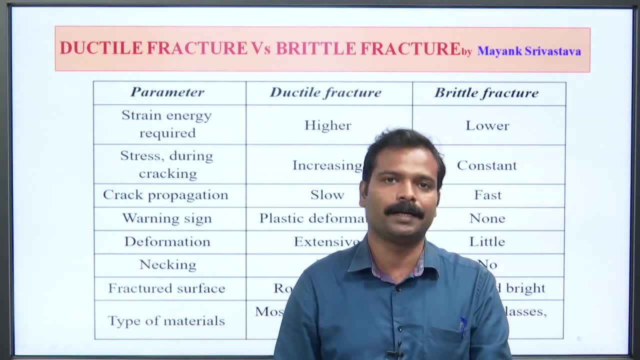 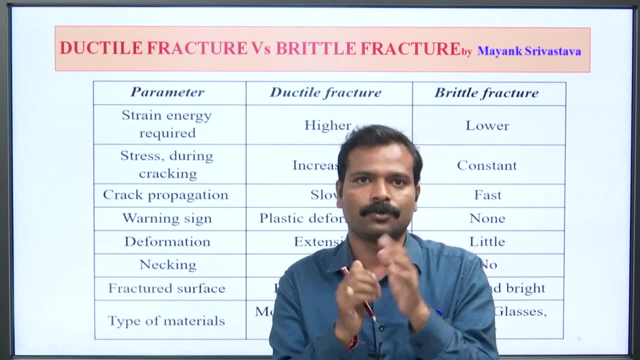 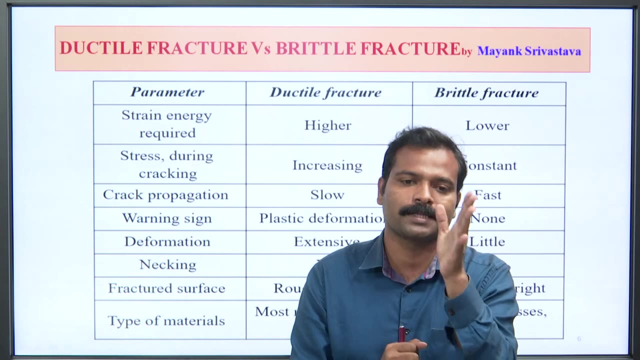 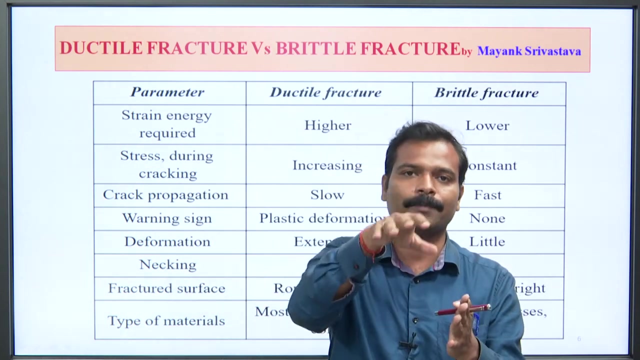 the term is warning sign, meaning that if there is ductile material, then or any material- if you think, give a sign before breaking that yes, we are going to break, then it is such a good, important factor of it. then in warning sign ductile fracture is plastic deformation, then here you get a warning sign. warning sign means if it is going to break, then it will show some impact on the surface that you will understand by looking at it that now we need to do regular maintenance. 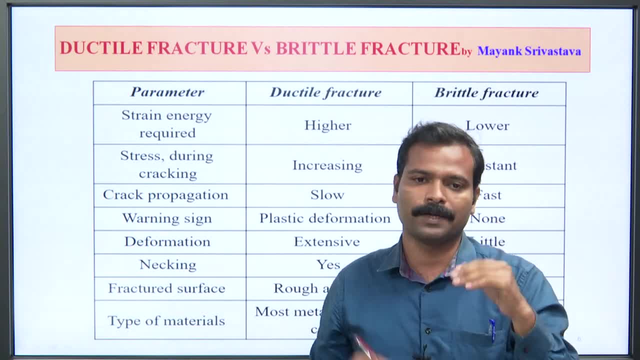 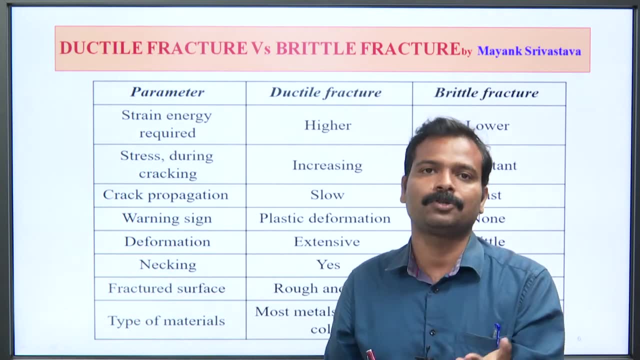 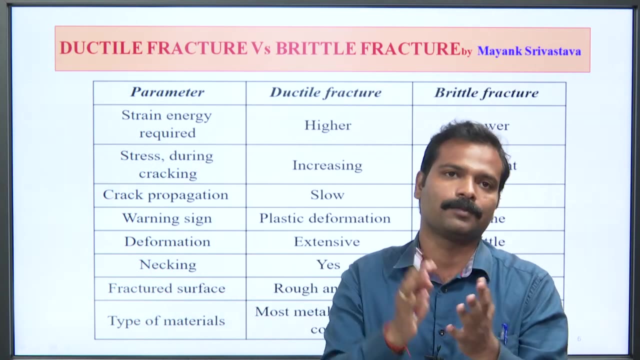 So that, for example, your propeller is soft or anything is movable or has any machinery parts in industrial use. if you do its proper maintenance, then on what basis do you do it? Because you know its life, how many days it will expire, how many days it will get worse. 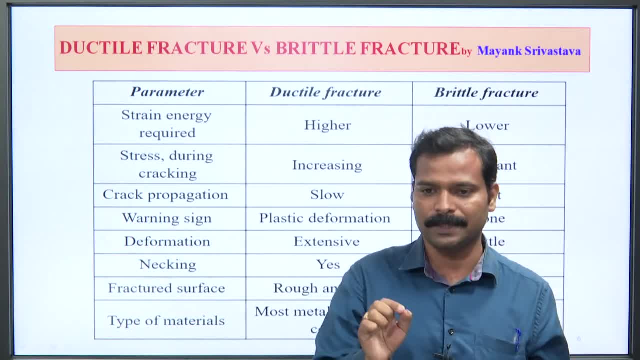 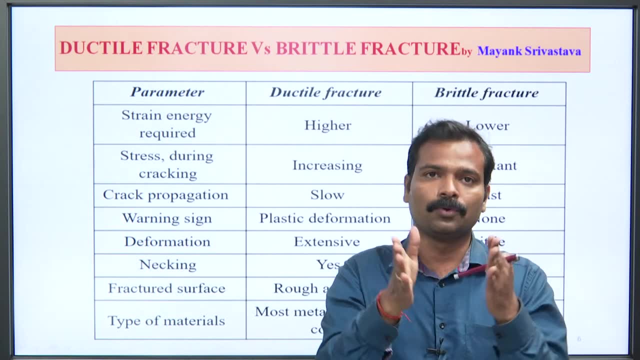 So if you get a warning sign, that means you get to know that, yes, this crack is coming in it now. why is the crack coming? because it is ductile material. now there is a crack in the ductile material, plastic deformation is happening. then it is so important. 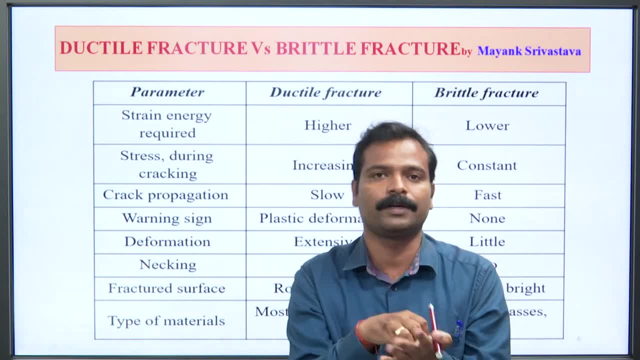 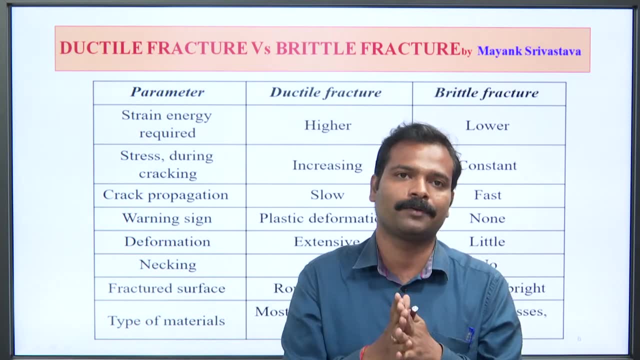 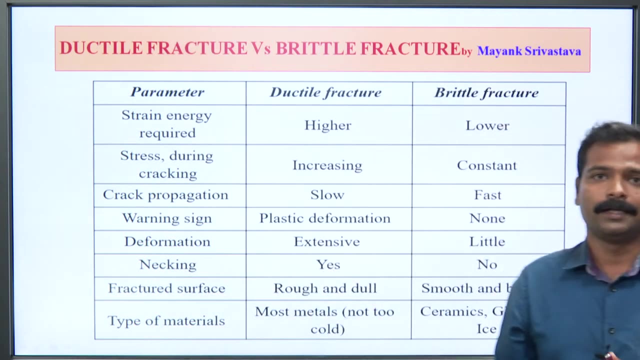 you will get a lot of benefit in selection and in case of brittle material, there is no sign of sudden failure. when there is sudden failure, you don't know when it will break, when you need to do maintenance, you don't know all these things. now comes the deformation. 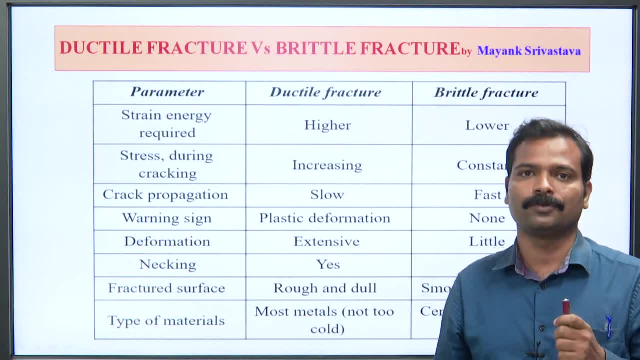 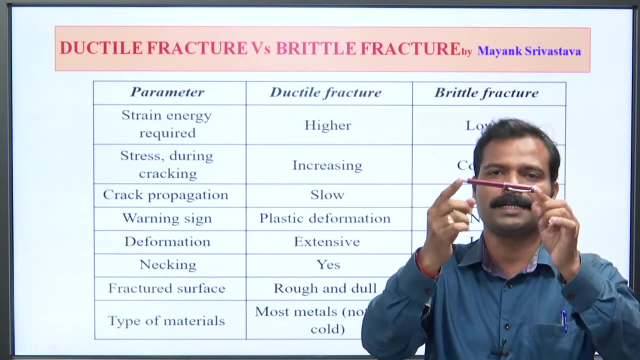 deformation is seen in ductile material. it is extensive. extensive means it is slow and it is very much deformation. if we talk about brittle, then it is less. if we explain you with an example, suppose this is a steel bar and in this bending stress is developing. you are applying bending force. 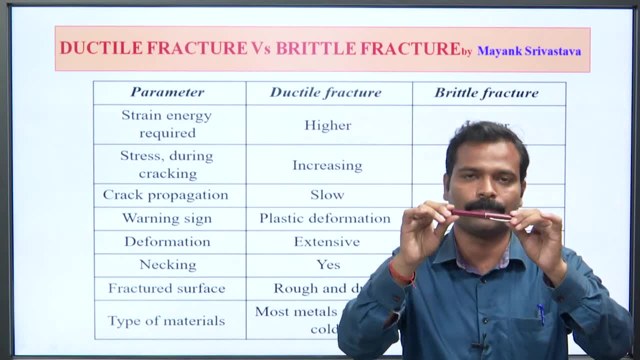 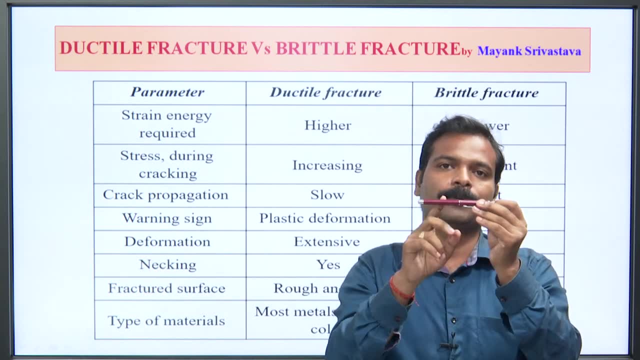 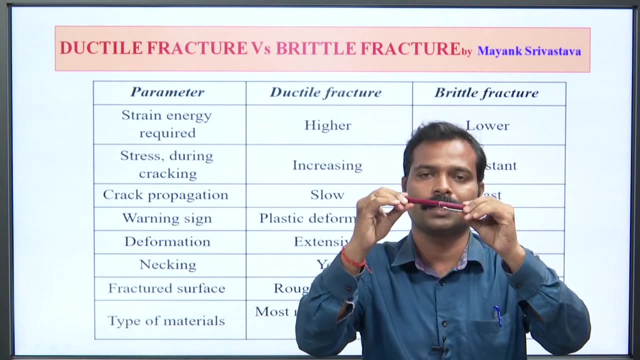 bending movement and in this bending stress is developing. and if it is written somewhere that this part has 500 MPa, is its limit now 500 MPa is the limit now you are bending it. then you applied 100, then 200 load, till then it will stand. 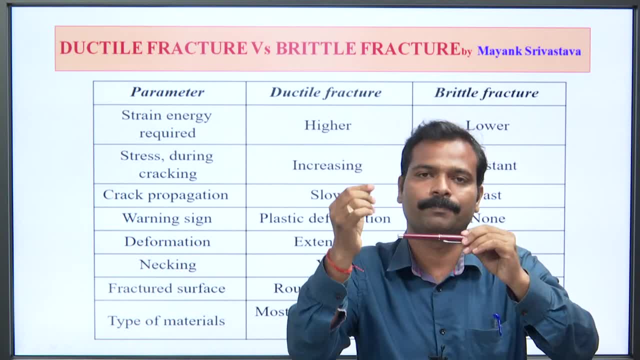 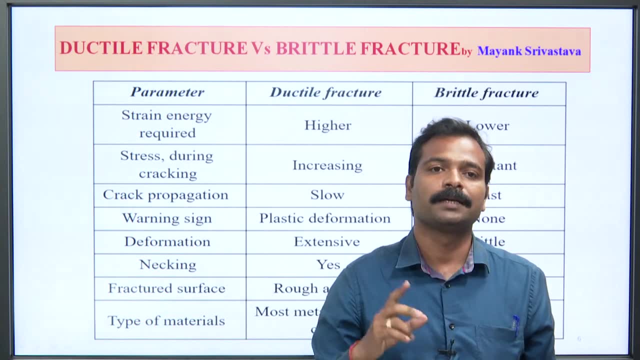 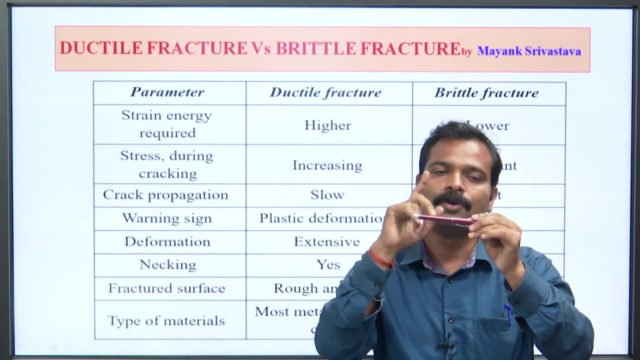 but as soon as you touch it above 499, touch 5- failure will happen. why it will fail? because bending stress is more than its limit. ok, bending stress, due to which bending stress is developing. it is more than its limit, so its color will be deformation. failure will happen. 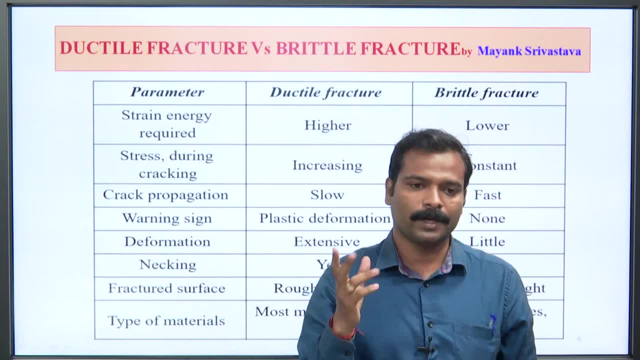 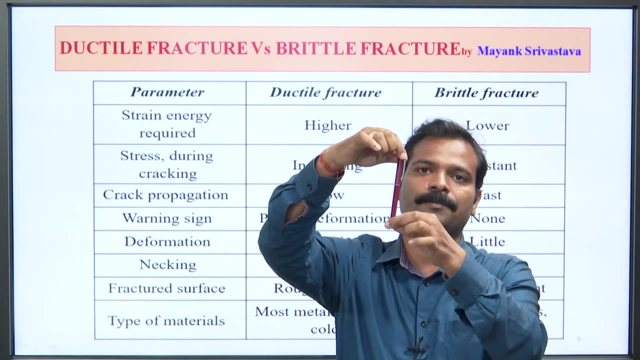 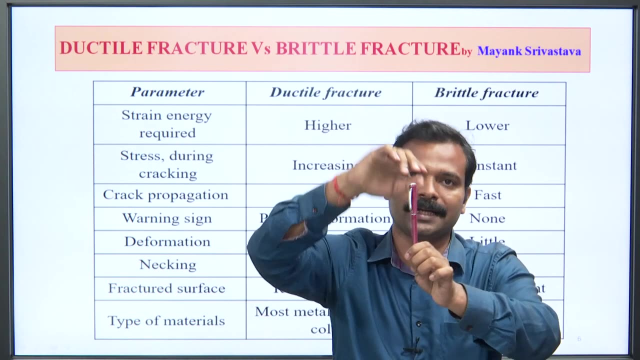 and if you talk about shear stress, what is shear stress? suppose this is a steel bar. now you apply torque in it. in the case of shear, you always apply torque. now you are applying torque in it. torque means you are bending it now as soon as you apply torque on it. 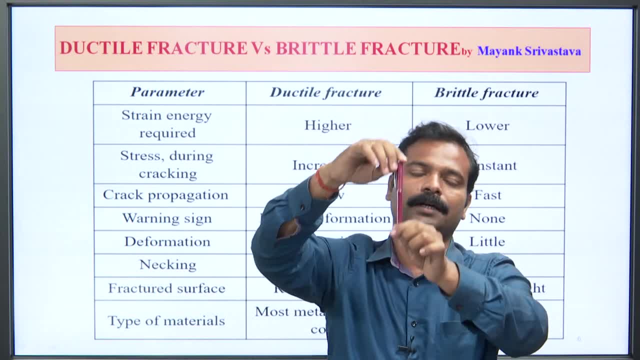 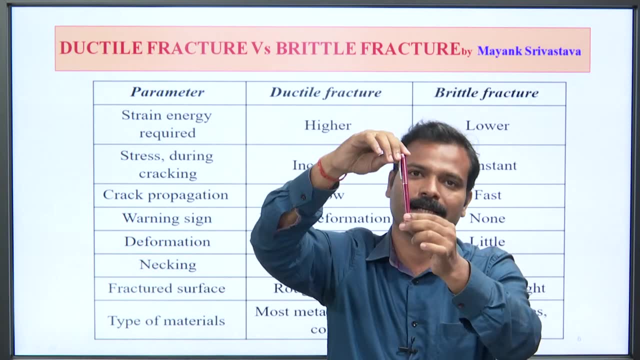 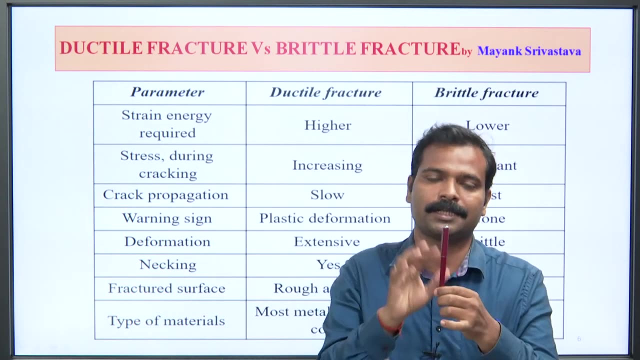 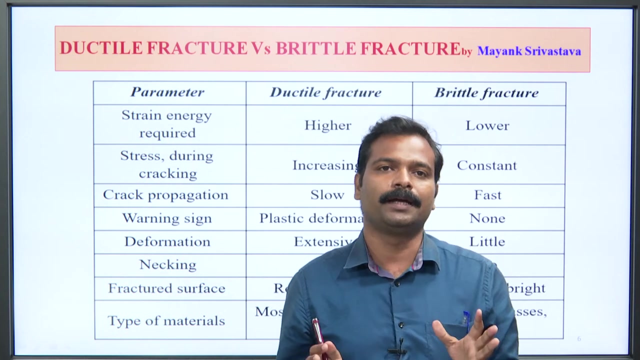 and suppose its limit is 200. now you apply torque of 50, then 100, then 120, then 130, then 145, then 149, then 120, and then 2 and 3 and 4 and 4 and 5 and 6. 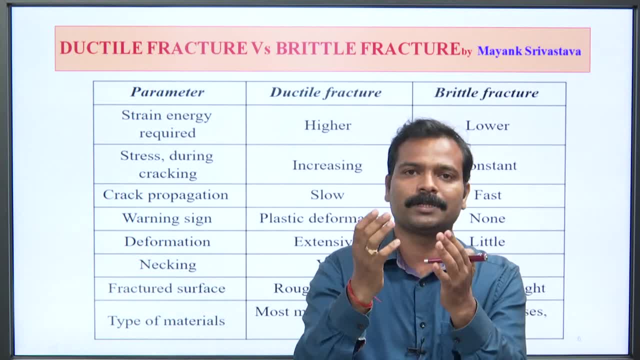 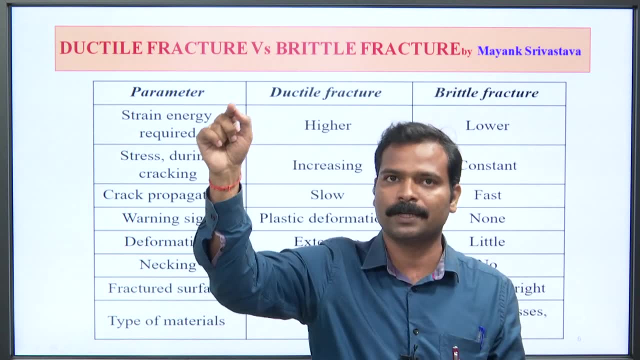 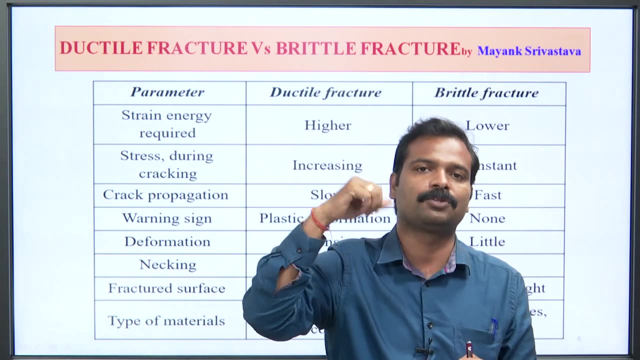 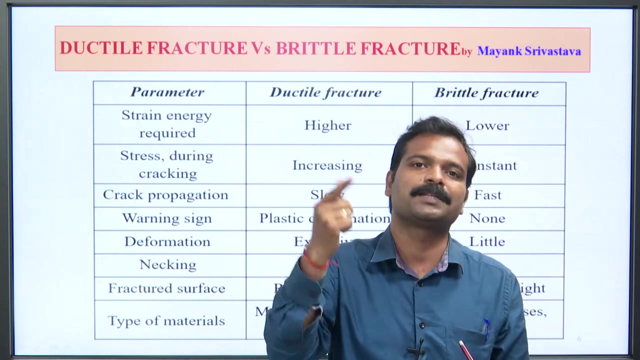 and 6 and 7 and 8 and 7 and 8 and 9 and 10. So in this way the ability to do stored energy is very less. it becomes brittle immediately. That is why it is more in strength, because it bears more stress, but deformation occurs very quickly in it. 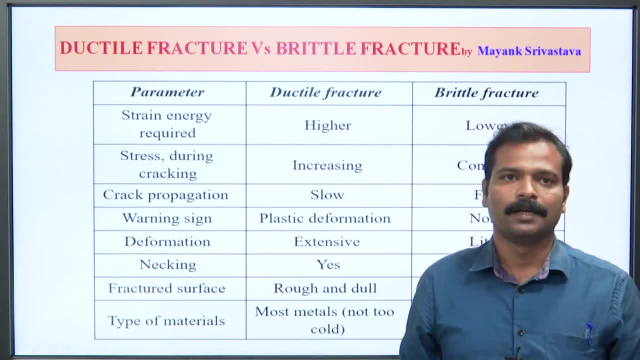 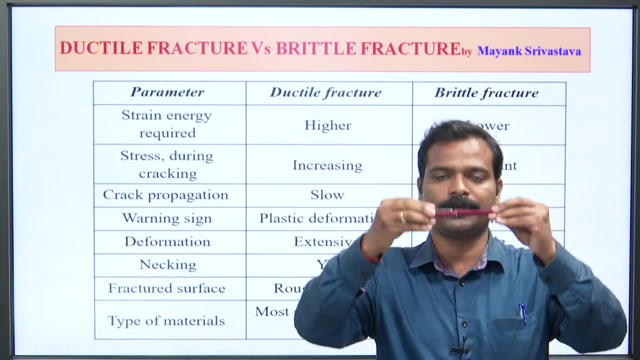 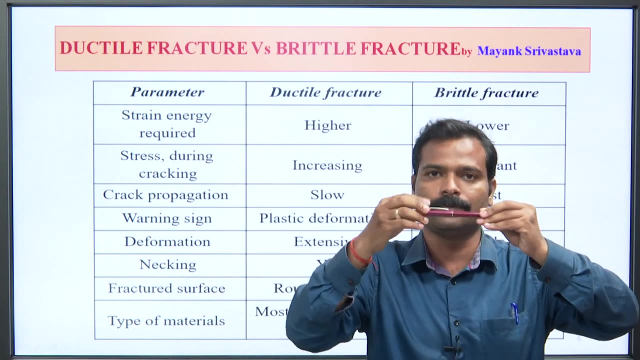 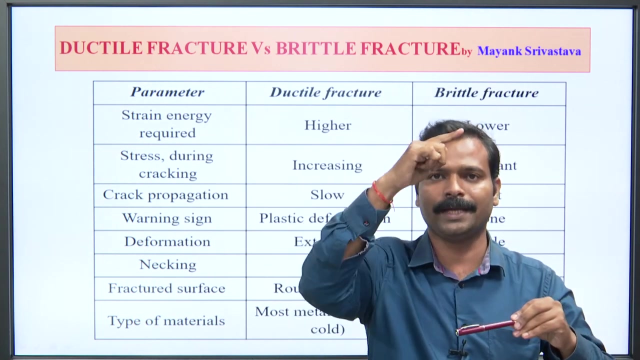 Now after that? next is your parameters necking. these are also important terms. in ductile material there is always necking formation. necking formation means if you are giving stress in it, it is elongated. for example, if there is something of D diameter now you have given tensile stress on it, load is applied, then tensile stress is developed. then what happens? from this center, your diameter starts to decrease. 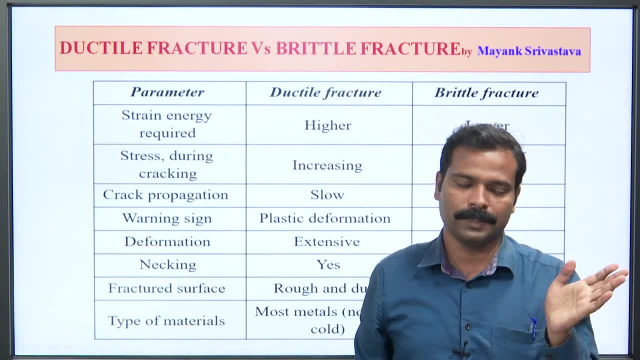 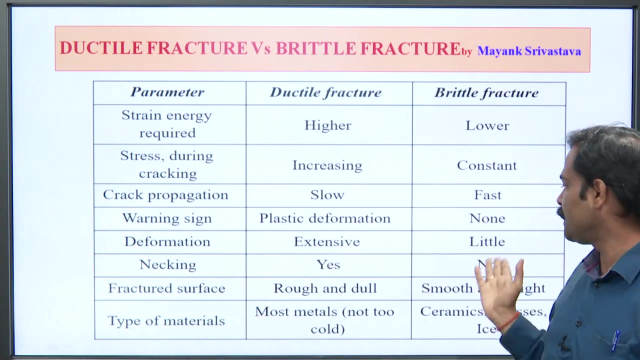 So one neck formation is formed. we will tell this in the next slide. so what happens in this? in the case of ductile, you will get necking. the properties of necking will be found in ductile. Why? because it follows the plastic limit. it goes up to the plastic limit, but this does not happen in brittle, which is written in you that there is nothing like this in brittle. 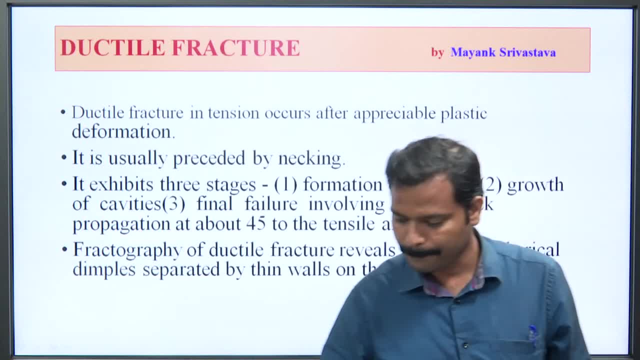 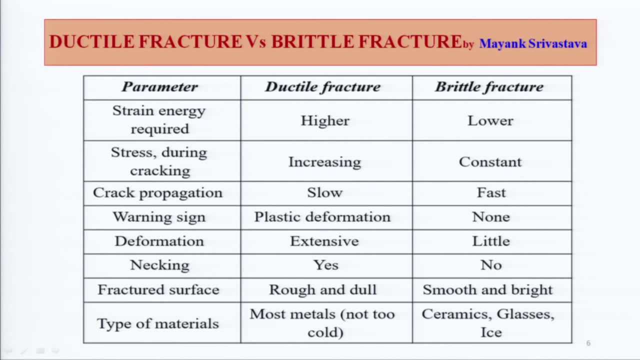 And if you look at its next parameters, if we talk about the fractured surface, then whenever your ductile material will be fractured from anywhere in two parts, then the surface that will come, the cut section that you will get, it will be rough and it will be dull. dull means there will be no signing in it. it will be dull and it will be rough. there will be no brightness. 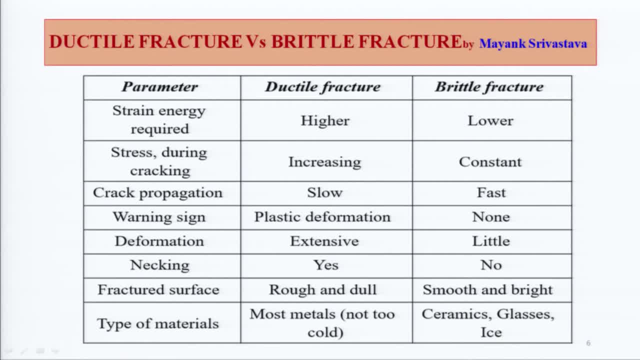 And in the case of this, if we talk about the case of brittle, then it will be like this: It is very smooth and your brightness is there In the last. if you talk about the types of material, if you talk about ductile material, then there are many examples of yours, like plastic or any of your aluminum. the best example is your gold. 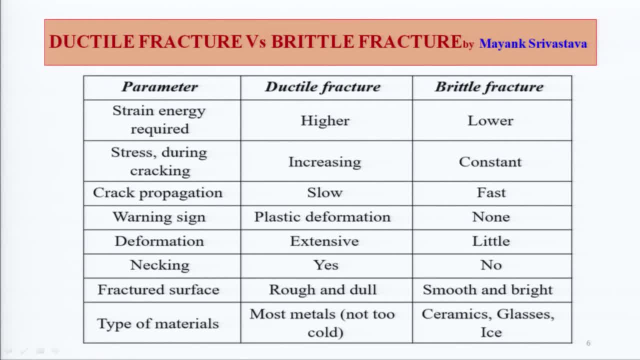 You can change it in wire form by pulling it, by giving tensile stress. But if we talk about the case of brittle, then what happens in brittle? there is ceramics and there are glasses, there are eyes. what happens in this? you do not have this atomic bonding. 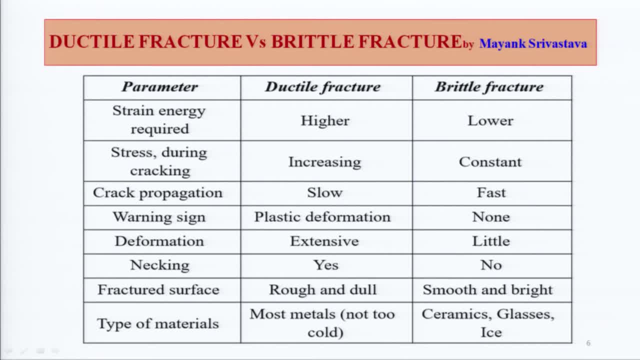 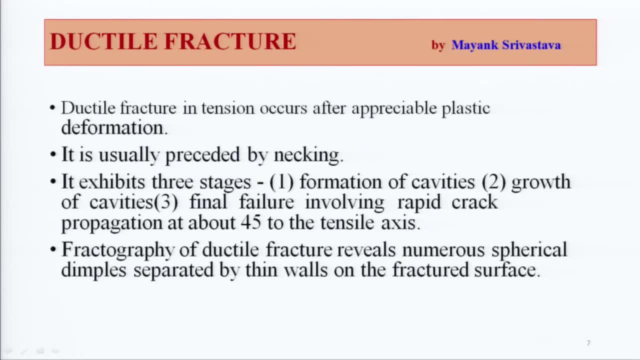 And after the elastic bond there is a sudden failure after the elastic limit. Now let's talk about ductile fracture. Intention occurs for the appropriate deformation. It is usually preceded by necking. It has three things. We will tell you one by one in the next. 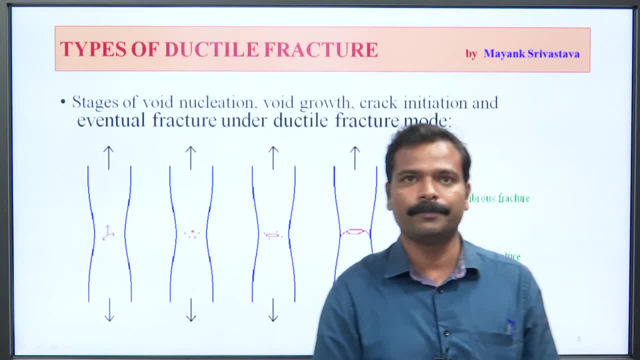 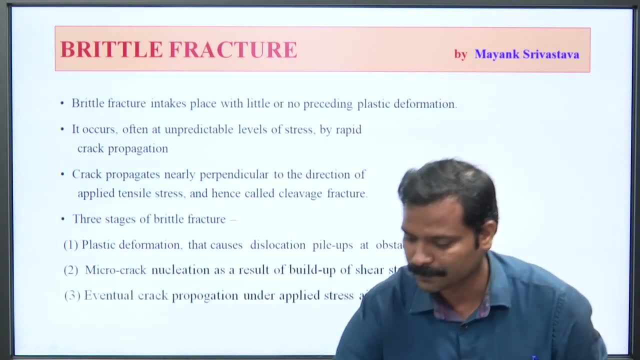 This is the main. What happens in this? What happens first? What is the first point? What is the first point? Suppose this is any of your bars. This is any of your bars given in the first. What is happening in this? 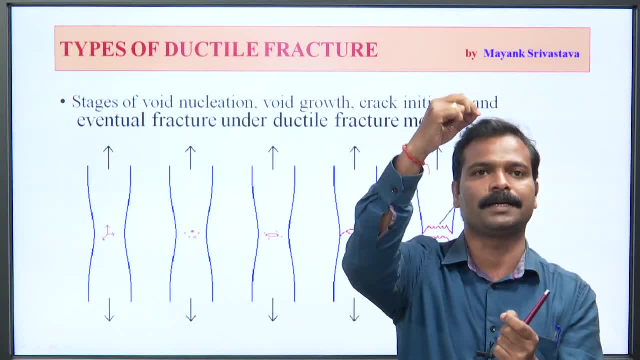 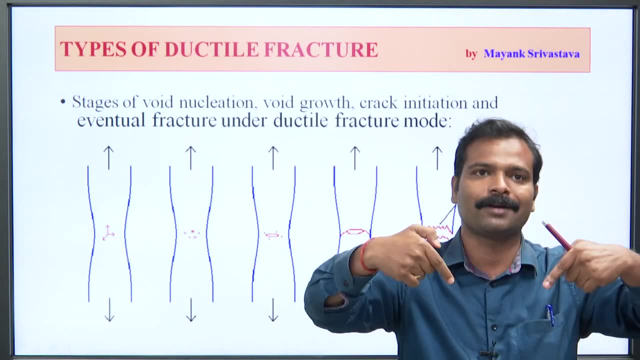 First of all, neck formation occurs. Now, if you give pressure from both sides, then internal stresses are developed inside and internal tensile stress is developed. then your diameter is decreasing and neck formation is happening. So this means that the material is in the tendency to break from the center, from here. 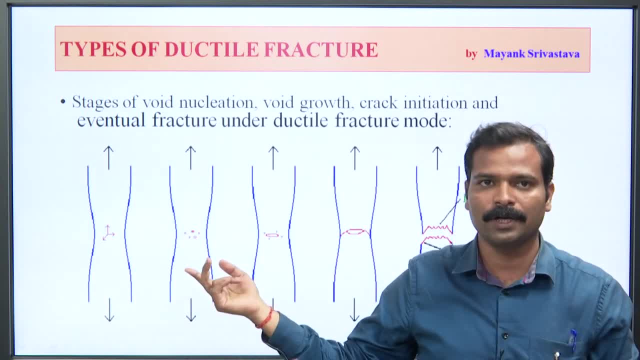 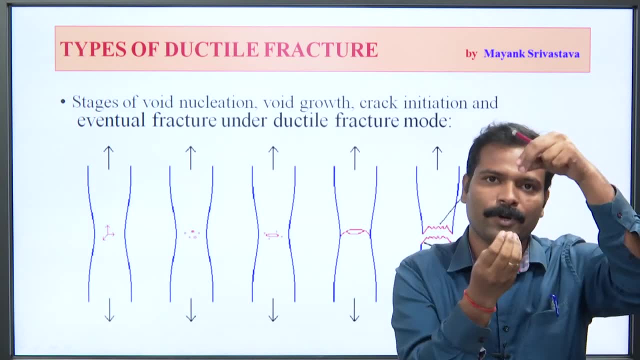 It is just starting now. What is written in the second phase? What happens? Cavity is formed. First of all, small cavity is formed. This is called voids. That means, if you give more pressure, then small pits are formed and cavity is generated. 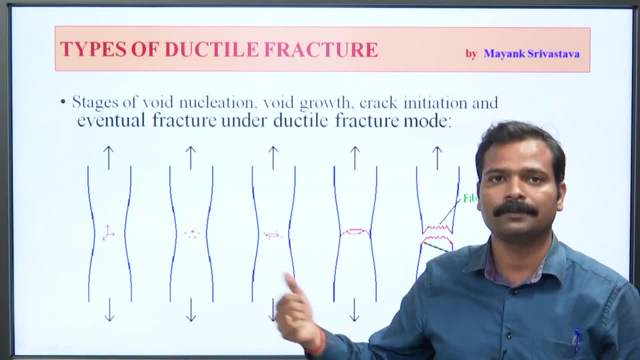 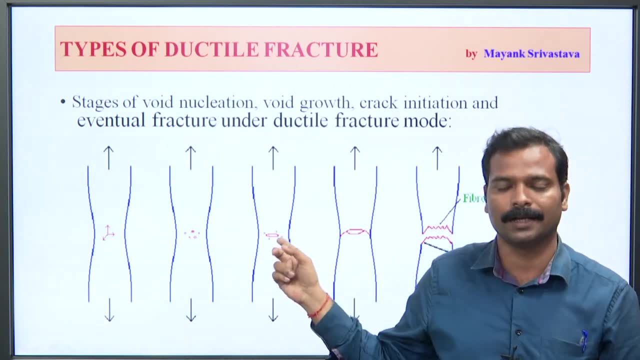 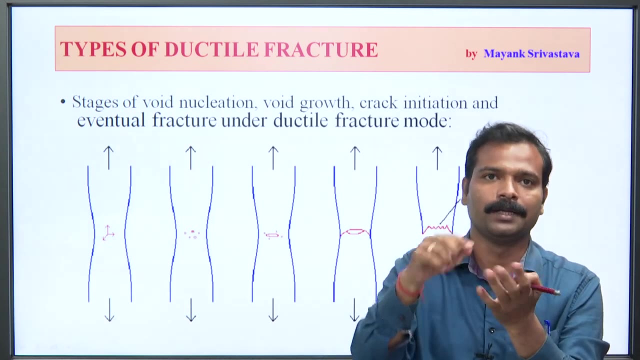 Now, after that, what is given in the third is your grain growth or your failure. after the cavity starts here, Growth starts here. Growth of cracks starts here, So this will always be at 90 degrees from the center, So growth will start here. 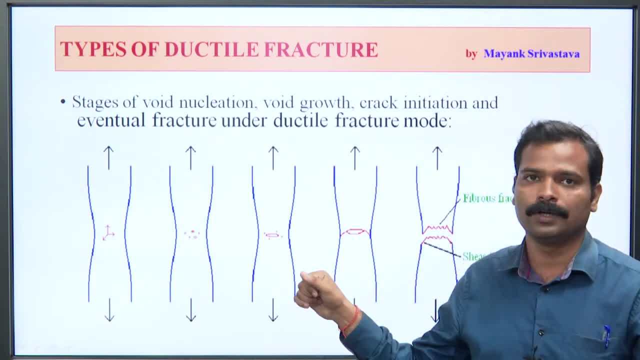 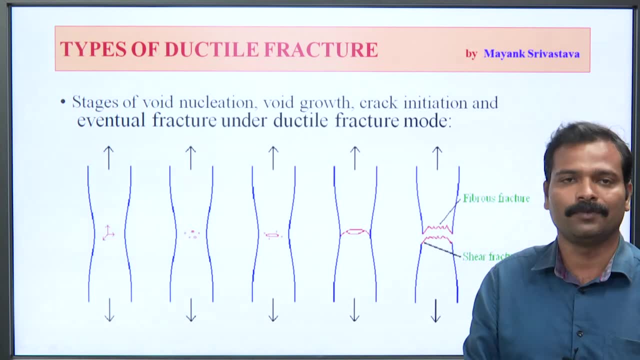 This is the third stage, And after that what is next? In the fourth figure you can see that it is at 45 degrees. Work is done at a 45 degree angle And here, whatever your growth is, it propagates. 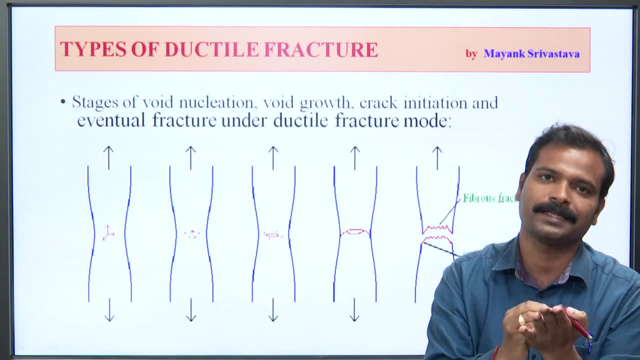 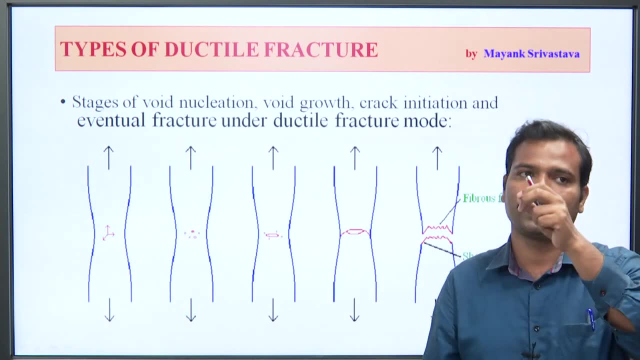 Whatever cracks come, it propagates at this stage. Propagate in the sense that it increases. That means if you give more pressure, it increases. Talking about the ductile case, it increased Now when it propagates more. So in the last the diagram that I told you before this, this is your last figure. 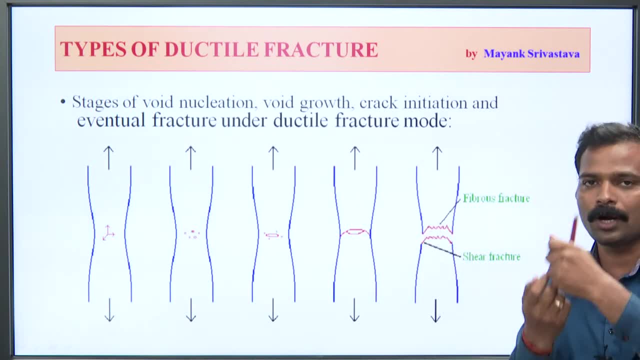 This is your fracture. What happens in the fracture? When you gave more pressure in it? then, after some time, after some period, what happens? It takes the shape of the cup and cone And from there your material breaks. So these are your five basic diagrams. 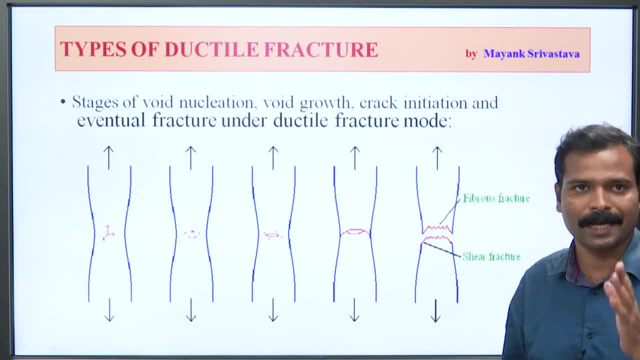 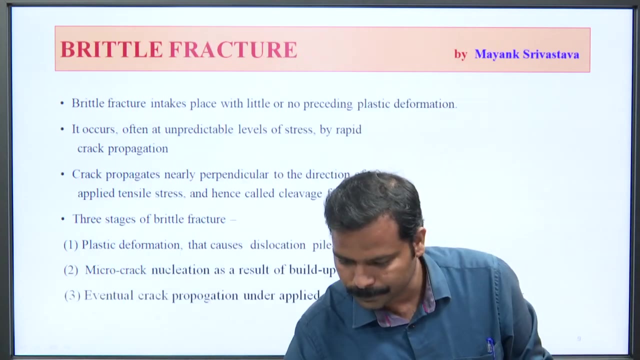 The first is your neck formation, The second is your cavity formation, The third is your crack grow up, And the third is your crack propagation. And the fifth one is your cup and cone fracture. So these are basically five types of fractures. Now let's talk about brittle fracture. 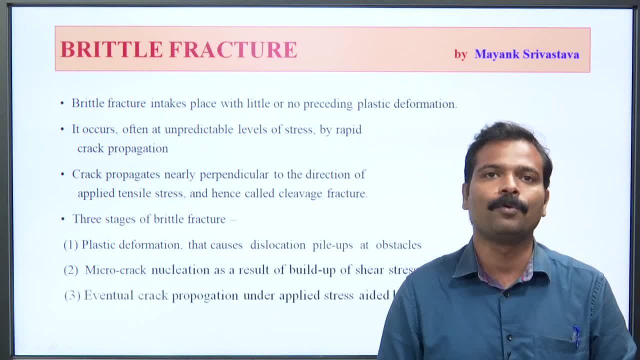 Brittle fracture intakes place with a little and no preceding plastic deformation. There is no plastic deformation in it. This fracture occurs with a little plastic deformation. It occurs often at appreciable level of stress by rapid crack propagation. That means the cracking process in it is very rapid. 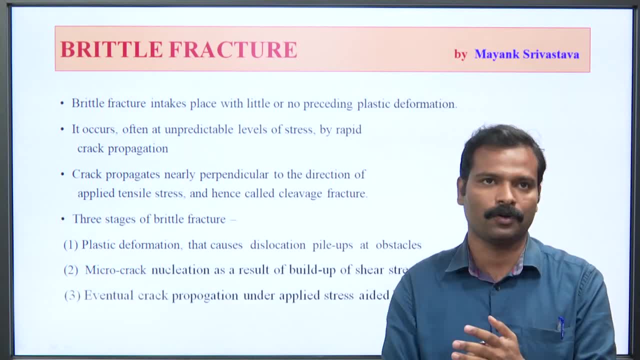 It is very fast. There is no time consumable in it because the plastic limit does not follow. After that crack propagates nearly perpendicular to the direction of applied tensile stress And hence called cleavage fracture, Which we have already told you in the previous slide. 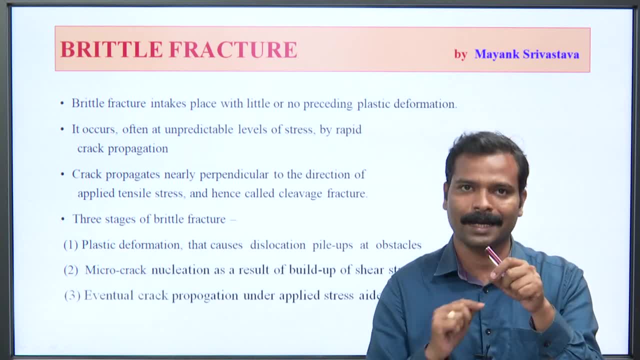 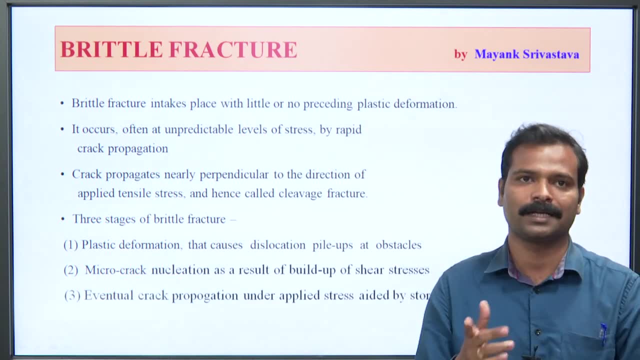 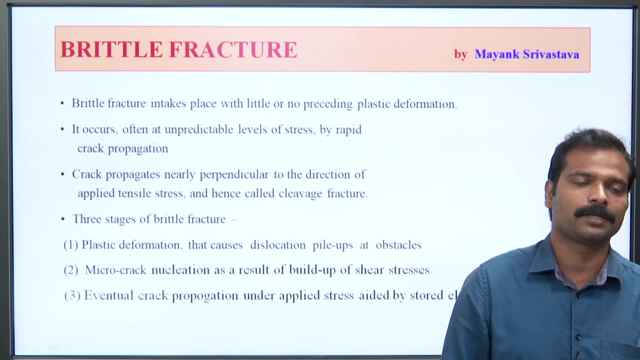 In this force is applied in perpendicular direction And crack is also called cleavage fracture, And this is three stages of brittle fracture. There are three stages of brittle. One is plastic deformation that causes dislocation or pile up obstacles, And second is micro crack. 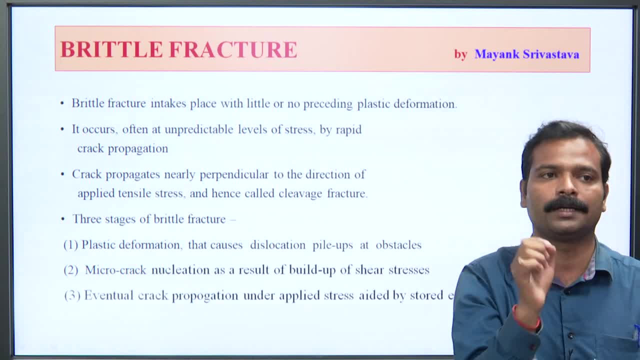 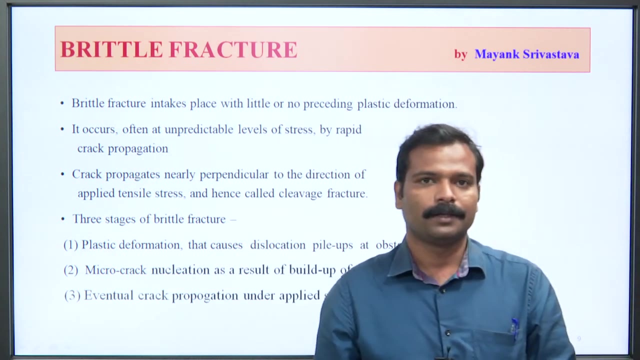 Micro crack means very small intensity Which is not visible at all, Nucleus of a result and build up of shear stress. This is because of shear stress. After that third is eventual crack propagation under applied stress added by stored. So this is the third step. 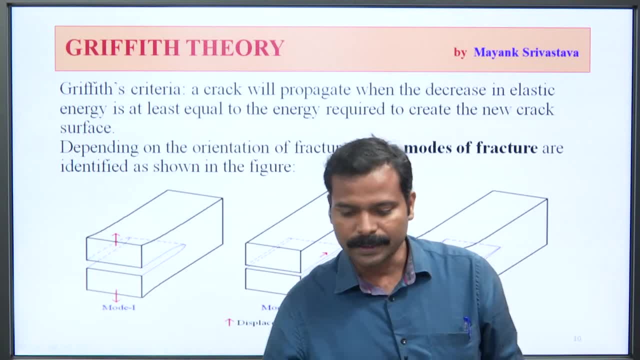 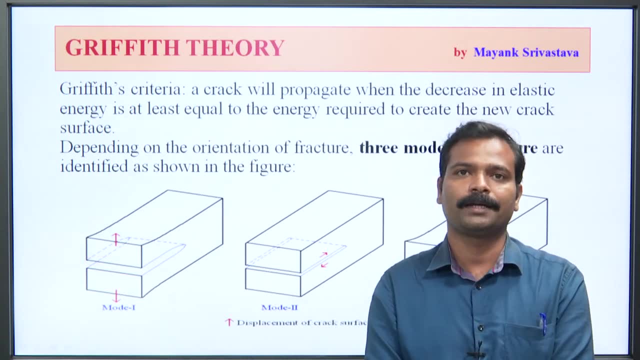 In this your Grifft criteria. is there Grifft theory? What is told in Grifft? That a crack will propagate when the decrease in elastic energy is at least equal to the energy required to create a new crack surface. What did Grifft tell?